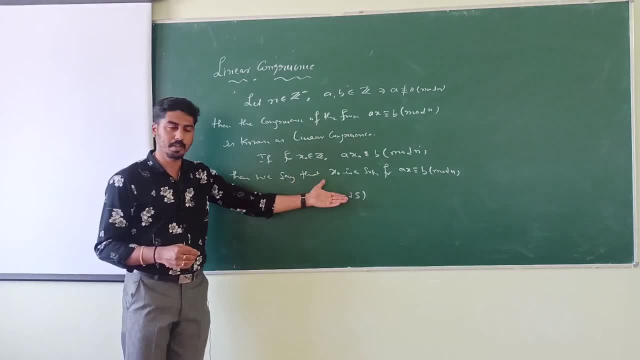 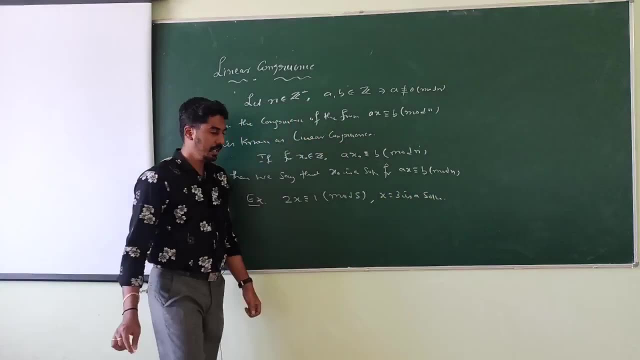 get 2 into 3 is 6,. 6 minus 1 is 5, which is a multiple of 5.. Therefore, x equal to 3 is a solution. Consider one more example: 2x congruent to 1. 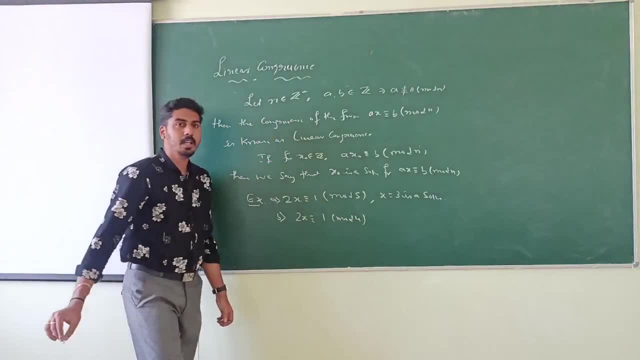 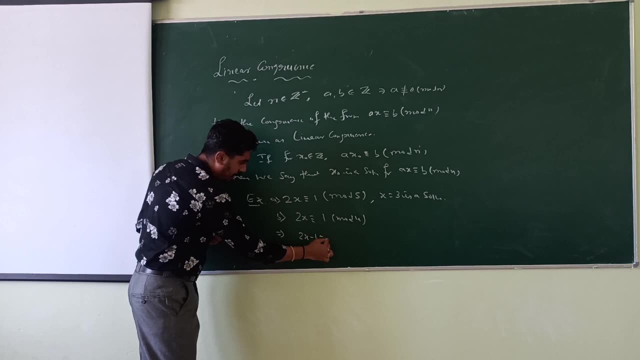 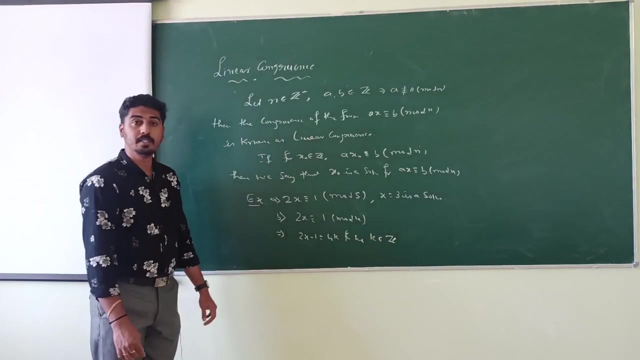 modulo 4.. By the definition of congruence we have: 2x minus 1 is equal to 4k. for some k belongs to z. This is not possible because the LHS is an odd number. RHS is an even number, So 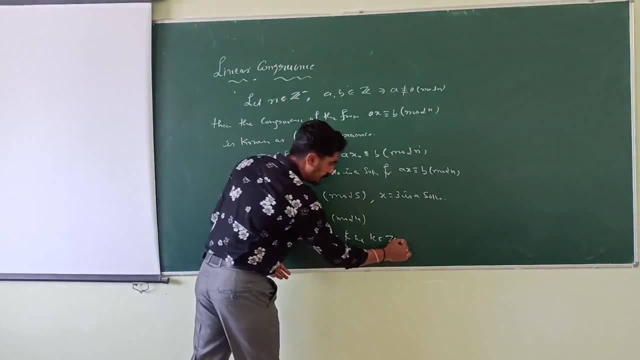 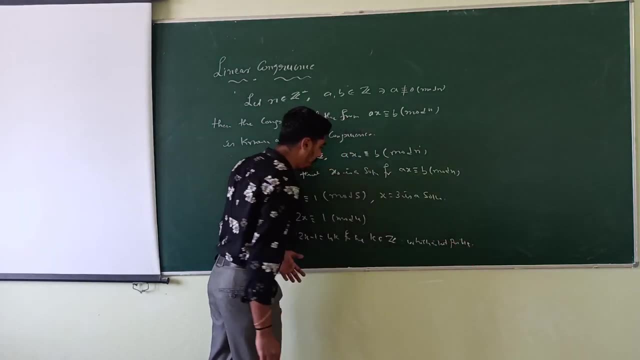 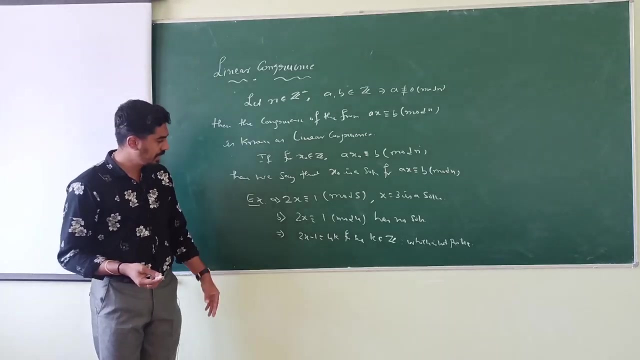 this congruence has no solution, which is not possible. Therefore, this congruence has no solution. So we have two examples. that first example: it has a solution, and second example: we do not have a solution. Now let us learn given 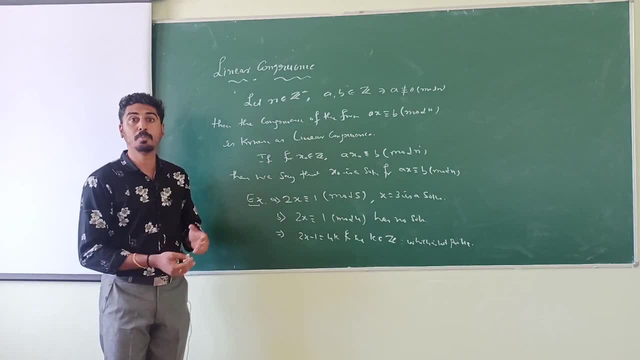 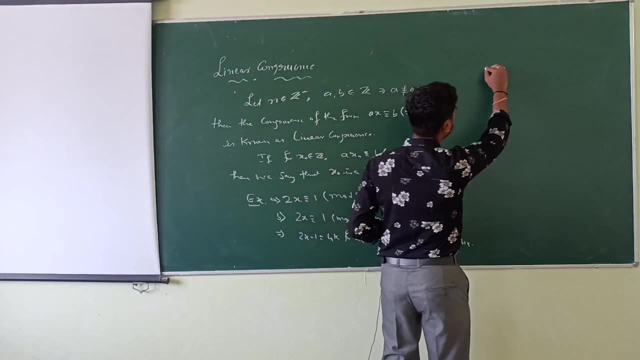 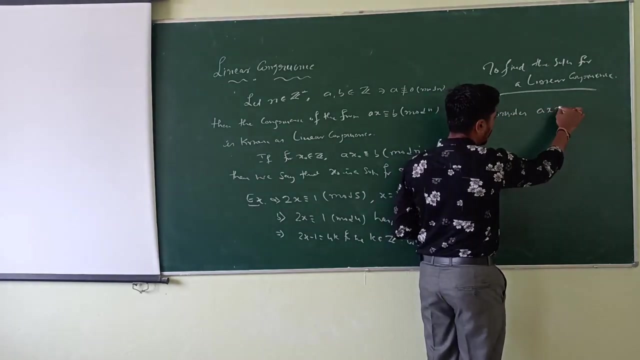 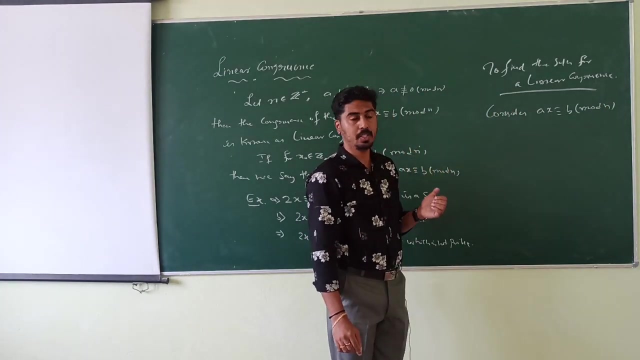 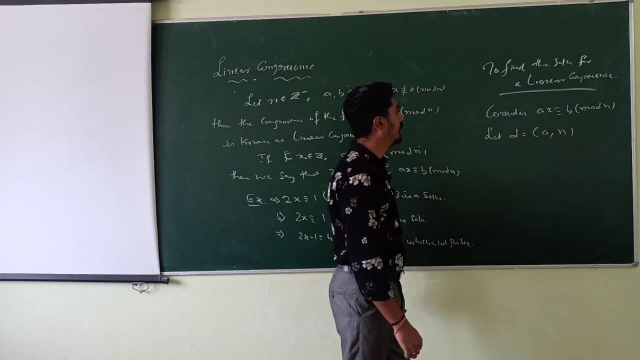 a linear congruence: when does solution exist and how many solutions exist and when does solution does not exist? To find the solution, first consider a linear congruence: A, x congruent to B modulo n, and let D be the GCD of A and N. Then we can show that this linear congruence 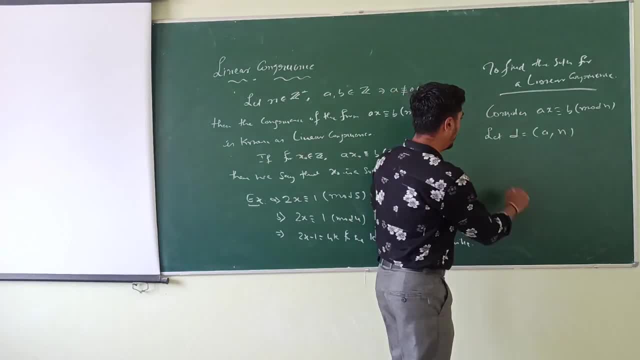 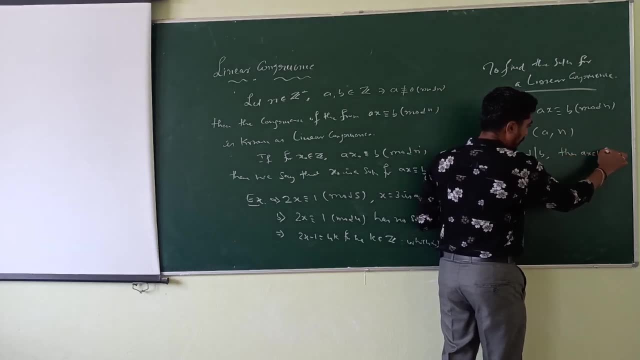 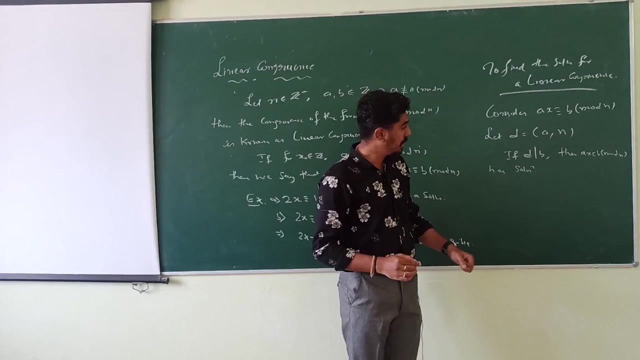 has a solution if D divides B. If D divides B, then A x congruent to B, modulo n has solutions. In fact, we can show that if D divides B, then this linear congruence has D incongruent solutions. In fact, has D incongruent solutions. 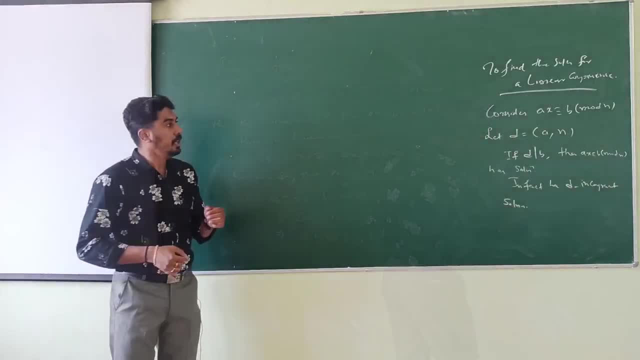 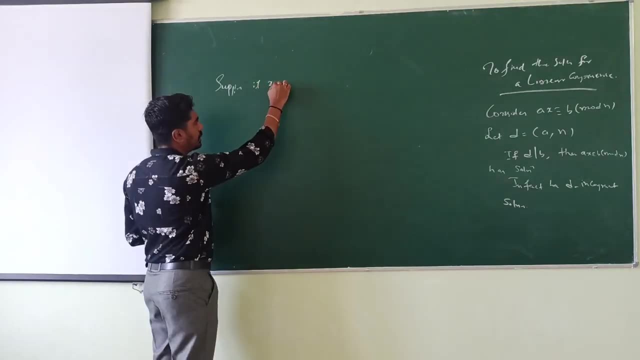 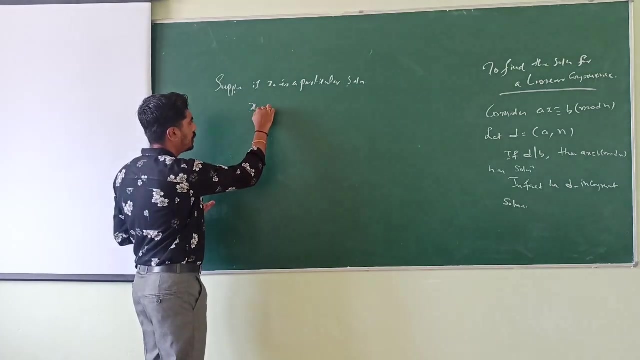 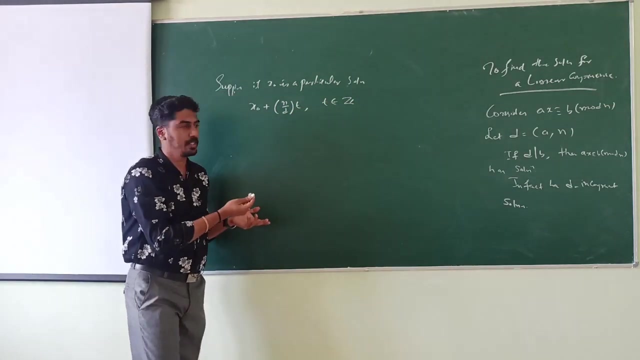 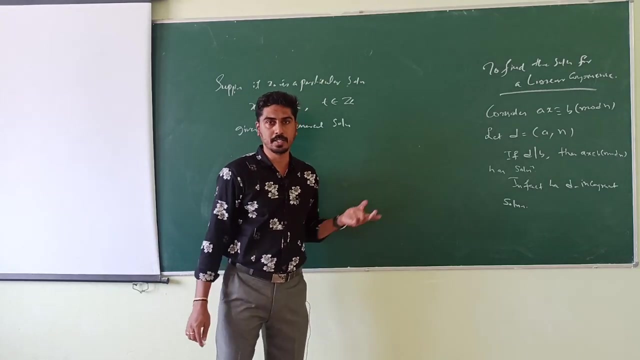 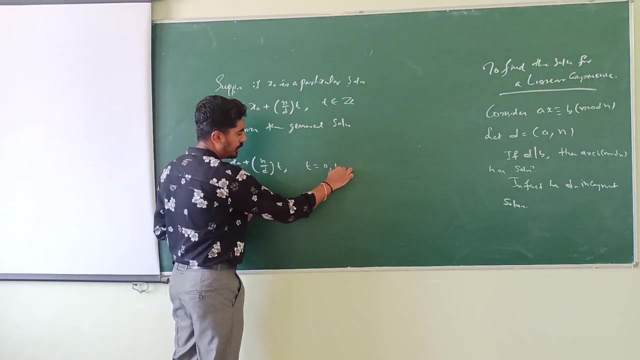 Suppose if x0 is a solution, suppose if x0 is a particular solution, then any integer of the form x0 plus n by D into T, for T belongs to Z is also a solution. So this gives the general solution. So for the incongruent solutions, x0 plus n by D into T, where T is equal to 0,, 1,, 2. 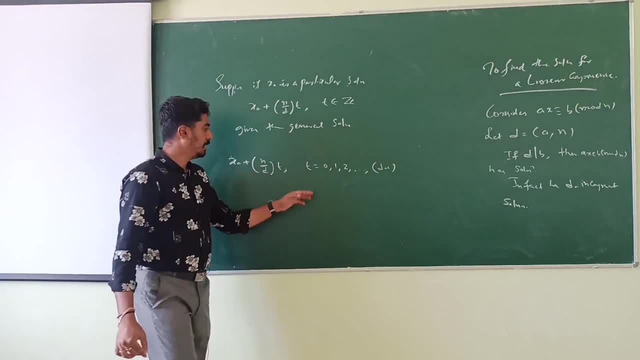 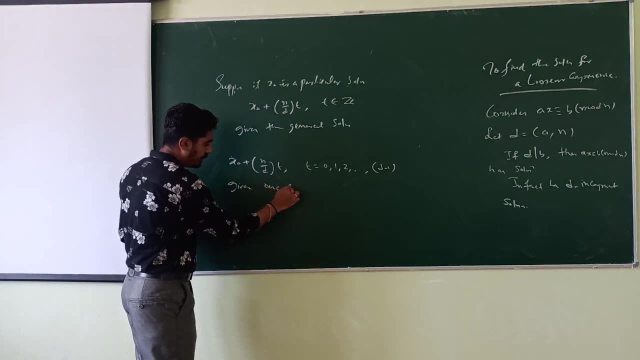 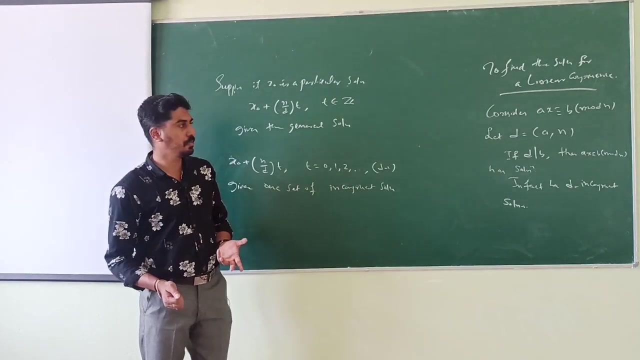 up to D minus 1, this set gives one set of incongruent solutions, One set of mutually incongruent solutions. So, given a linear congruence, first we need to find out the GCD of A and N. 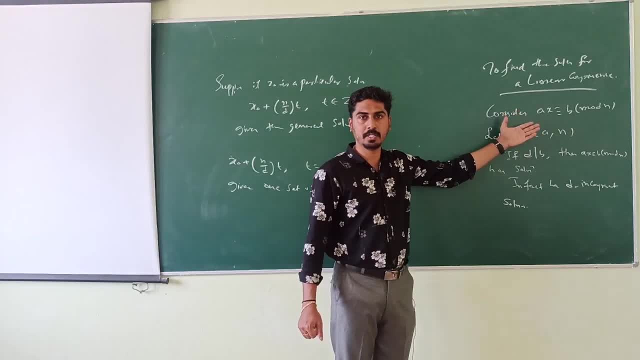 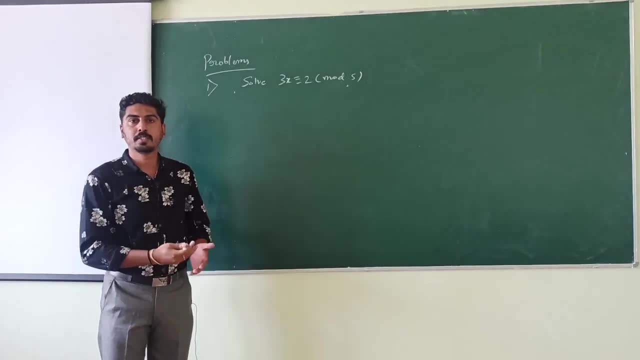 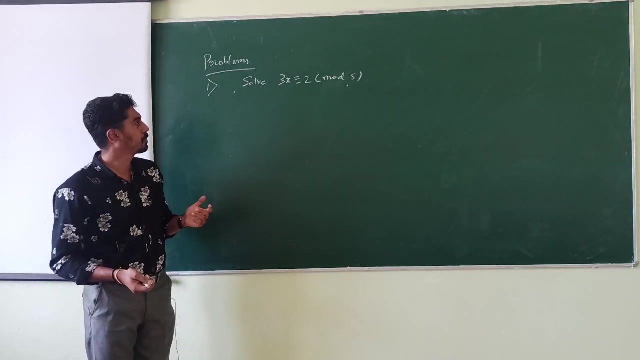 D. If D divides B, then it has a solution. In fact, D incongruent solutions. If D does not divide B, then it has no solution. Now let us consider some problems on linear congruences. Solve 3x congruent to 2 modulo 5.. First let us check whether this congruence 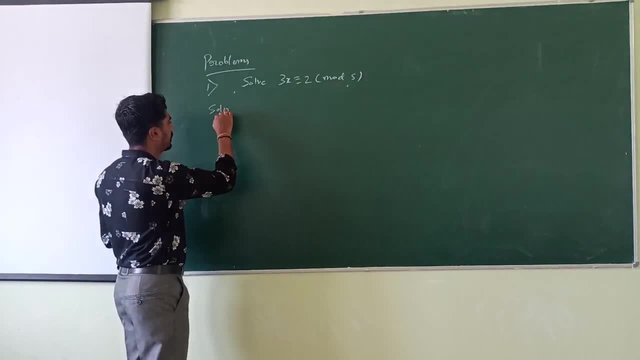 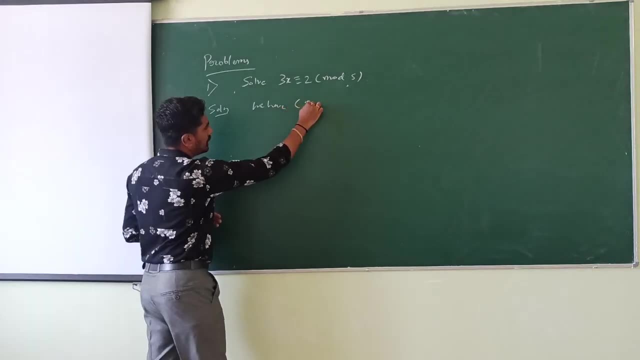 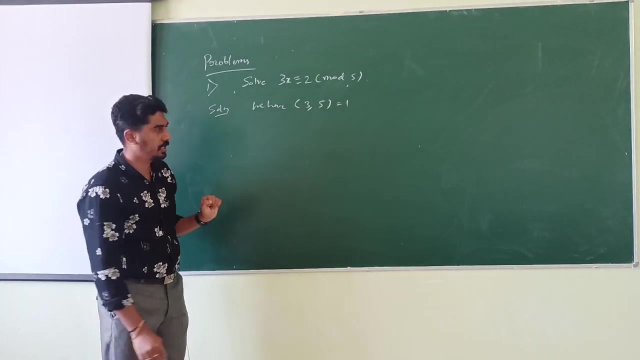 has a solution or not? Solution: First find out the GCD of 3 and 5.. We have 3, the GCD of 3 and 5 is 1.. So the given linear congruence has a unique solution. This implies given: 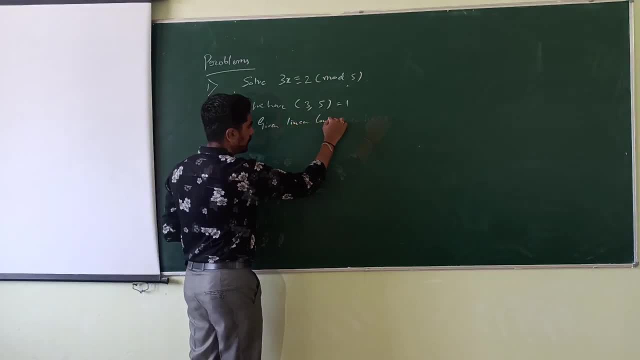 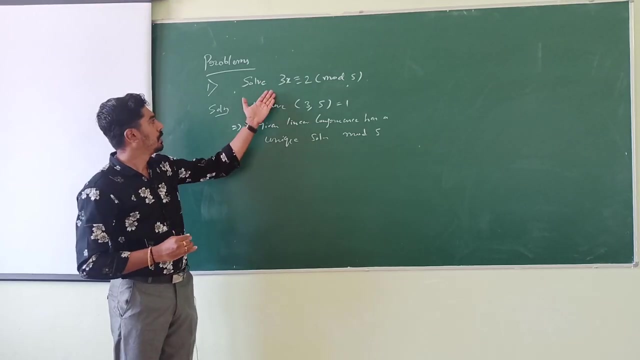 linear congruence has a unique solution: modulo 5.. To find out the unique solution, we can use the inspection method. If I put x equal to 1,, 3 minus 2 is 1,, which is not a multiple of 5.. When I put x equal to 2,, 3 to the 6,, 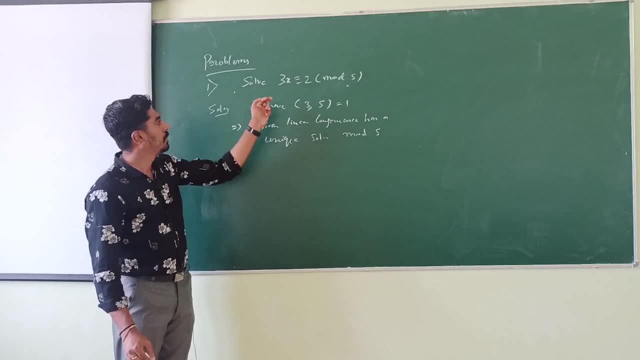 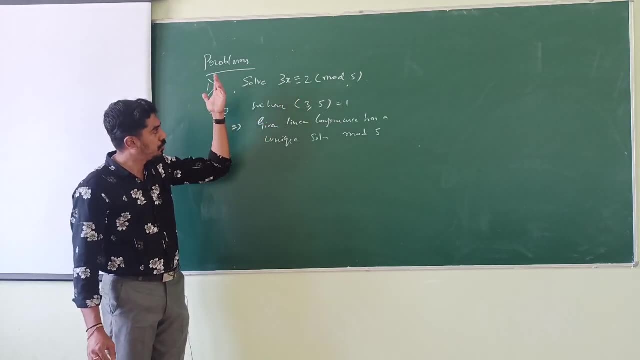 6 minus 2 is 4,. 4 is not a multiple of 5.. When I put x equal to 3, 9 minus 2,, which is 7, is not a multiple of 5.. Therefore, 3 is not a solution When I put x equal to 4,. 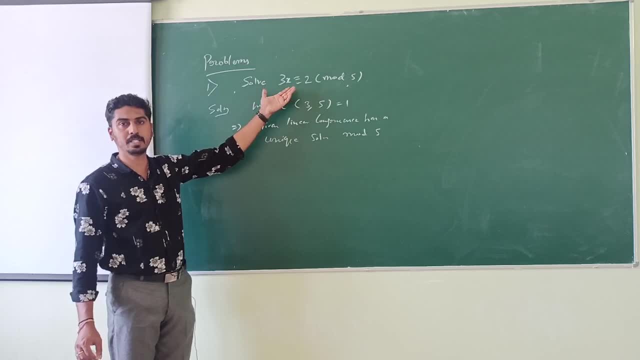 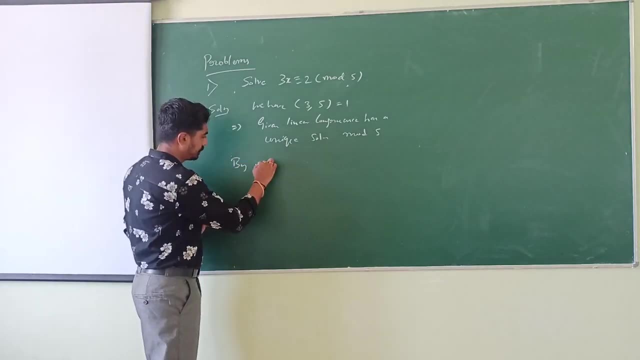 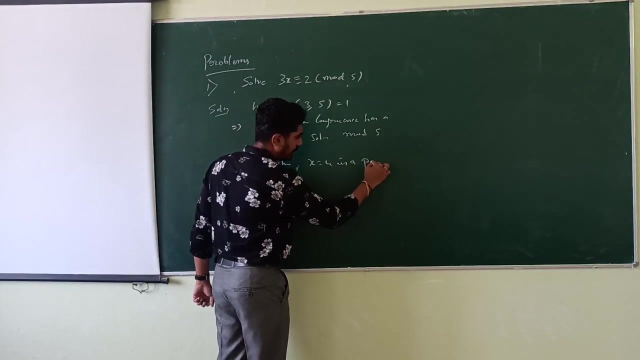 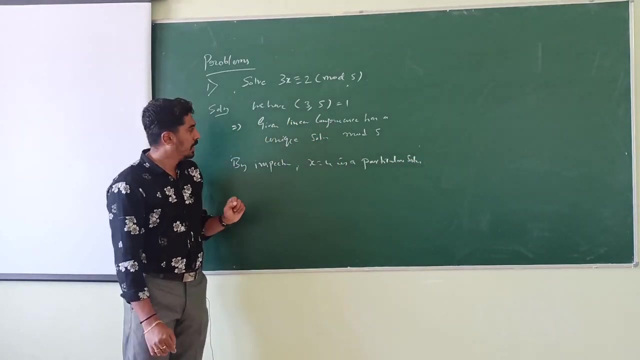 I get 3 into 4 is 12,. 12 minus 2 is 10, which is 5.. Therefore, 4 is a particular solution By inspection. x, equal to 4, is a particular solution or unique solution, modulo 5.. So the general solution is given by, therefore, 4 plus 5t. 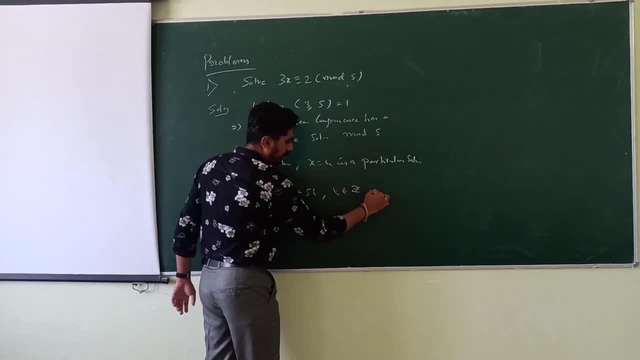 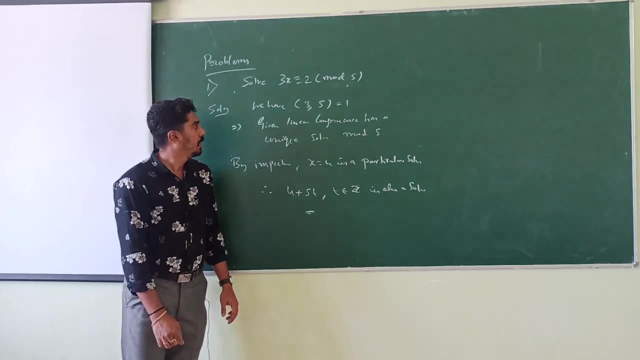 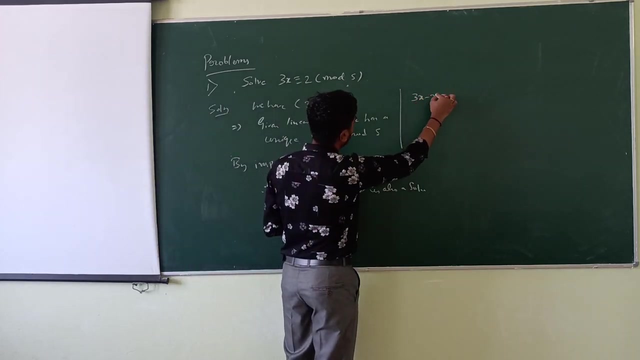 for all t belongs to z. This gives the general solution. When it is difficult to find out the solution by inspection, we can solve this: If 3x is congruent to 2 modulo 5, then 3x minus 2 is equal to 5k for. 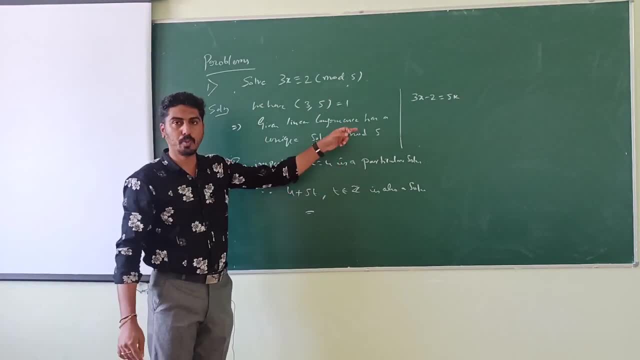 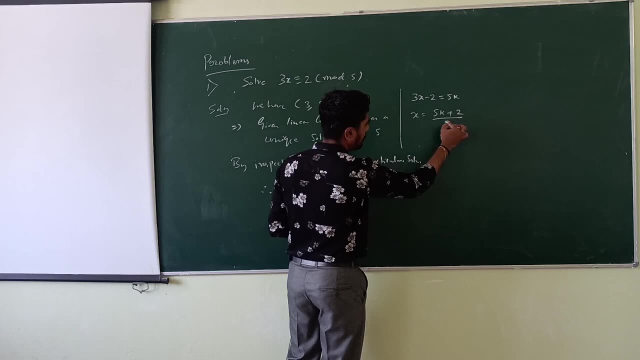 some k belongs to z, So solve this for x. I get: x is equal to 3x, minus 2 is equal to 5k plus 2 divided by 3.. Now substitute the values for k, k equal to 0,, k equal to 1 and. 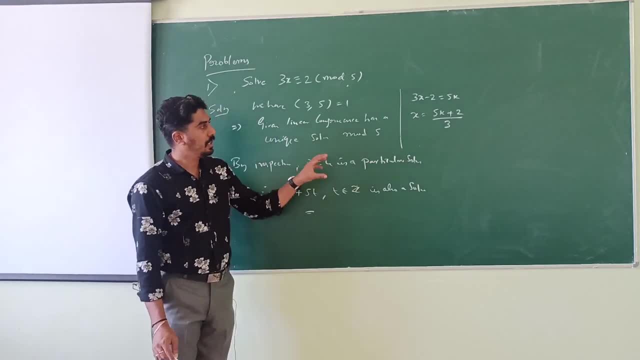 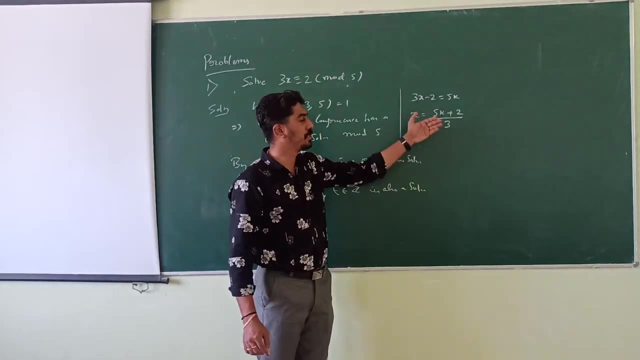 k equal to 2 and so on. If we get an integral value, that will be a solution. For k equal to 0, we get 2 by 3,, which is not an integer. For k equal to 1,, we get 7 by 3,, which is. 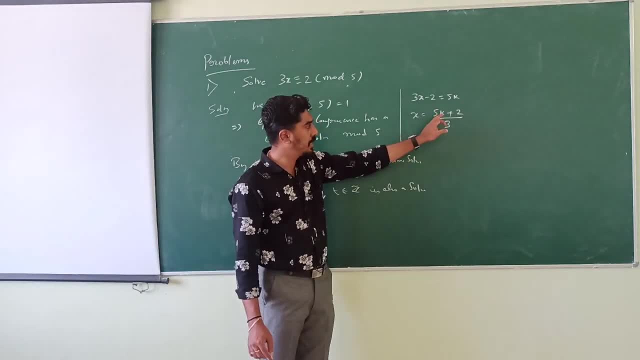 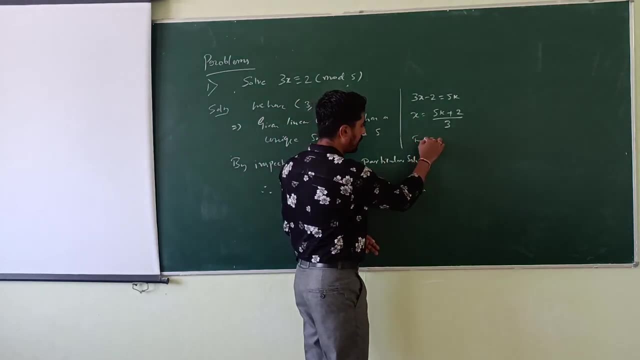 also not an integer. When I put k equal to 2,, I get 12 by 3, which is 4, is an integral solution. For k equal to 2,, we get an integral value: x equal to 4.. Therefore, x equal to 4 is a. 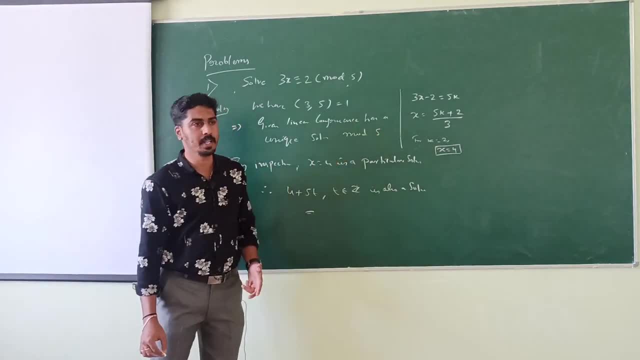 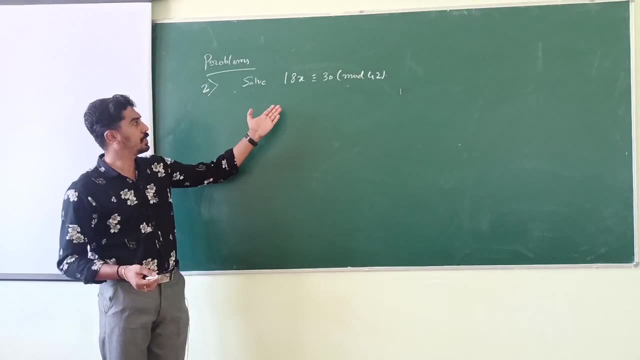 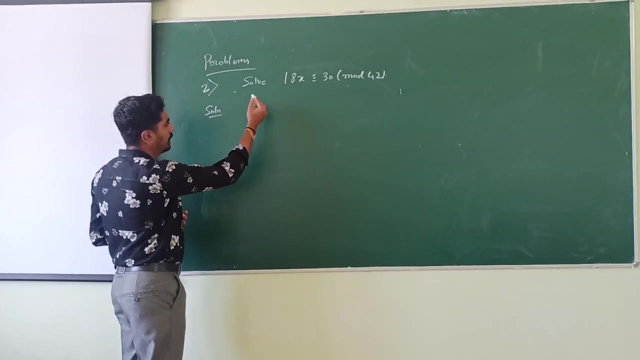 particular solution. This is another method of finding the solution: by inspection. Now consider one more problem. Solve 18x, congruent to 30 mod 42. First let us check whether this linear congruence has a solution or not. Find out the gcd of 18 and 42. The 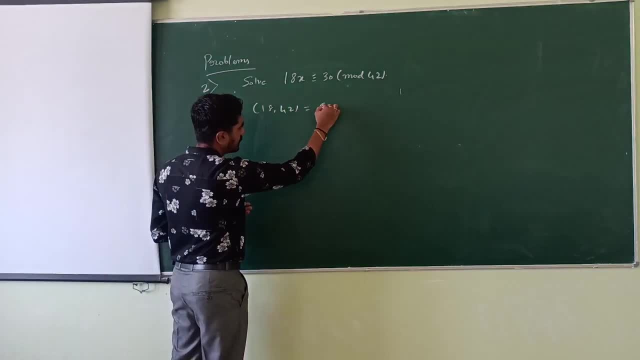 gcd of 18 and 42 is a solution. So let us find out the gcd of 18 and 42.. So let us find out the gcd of 18 and 42.. There, the gcd of 18 and 42 is a 6.. Also, we know that. 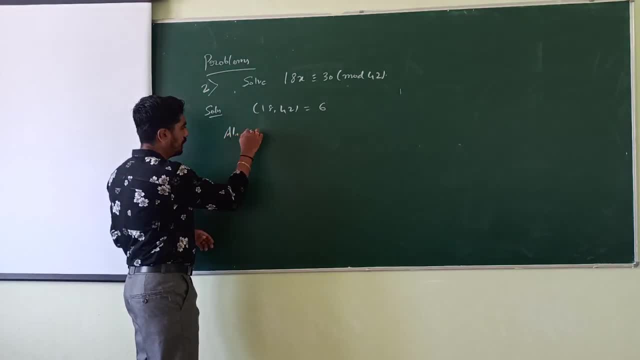 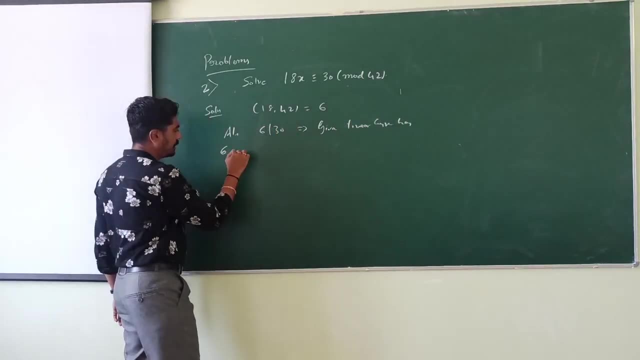 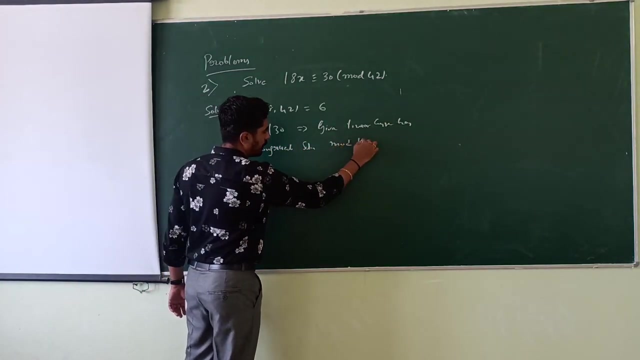 6 divides 30.. Also, 6 divides 30 implies the given linear congruence has six incongruent solutions: modulo 42.. As it has length 6, we need this solution: 1 from" C equals 1,. 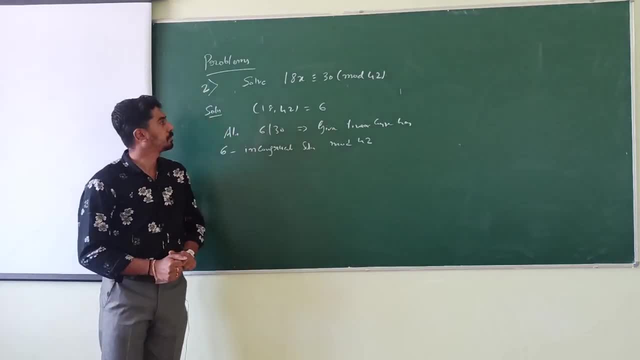 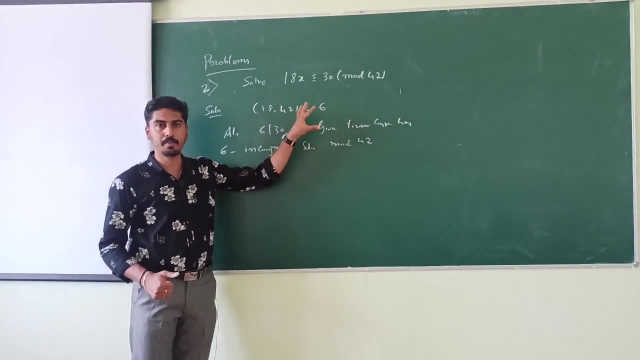 from mod et times 2.. Another example Now in this case: here we should find out a solution First we need to find out the a solution by inspection. But here, in this case, it may be difficult to find out the solution. 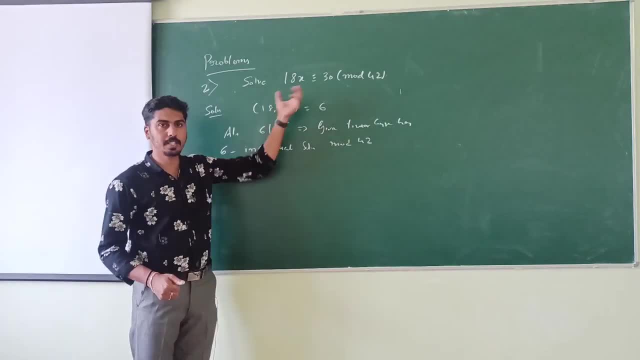 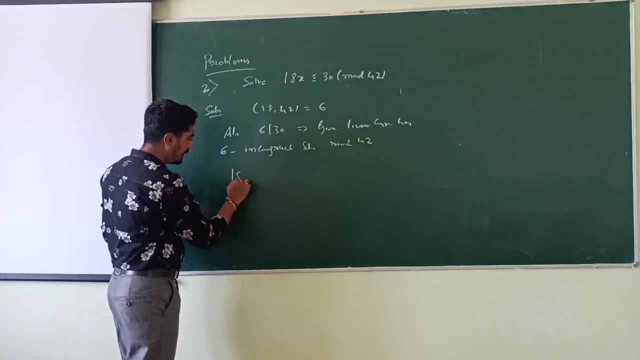 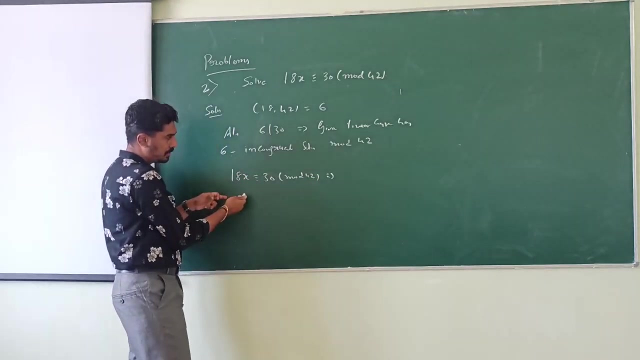 by inspection. So we can deduce this linear congruence by dividing throughout by the GCD 6.. This can be written as: 18x is congruent to 30 mod 42 can be reduced to 18 by 6, which. 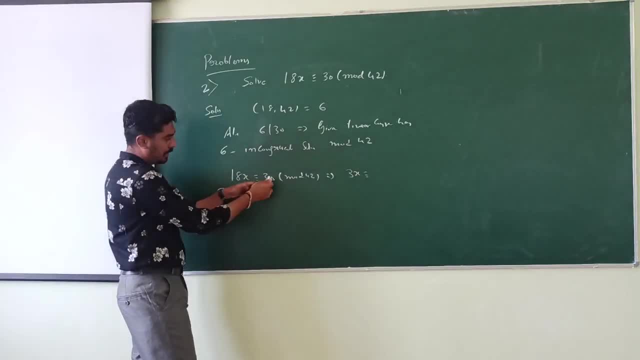 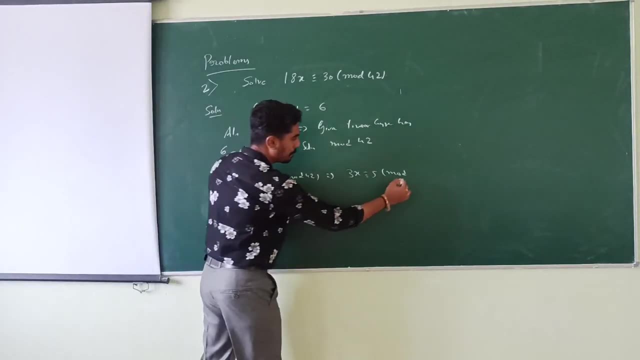 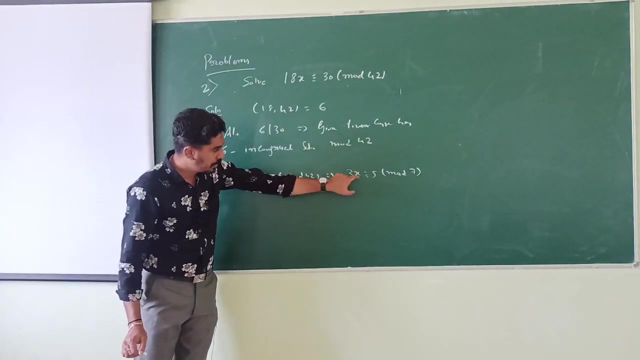 is 3x, is congruent to 30 by 6, which is 5, modulo 42 by 6, which is 7.. These two congruences are entirely different congruences, but the solution of this congruence is also a solution. 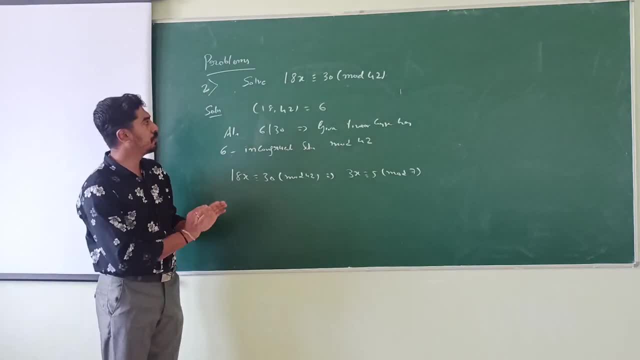 of this congruence. First, we need to find out a solution by inspection. So we can use this congruence, which is simpler than this congruence. So we can use this congruence, which is simpler than this congruence. So we can use this. 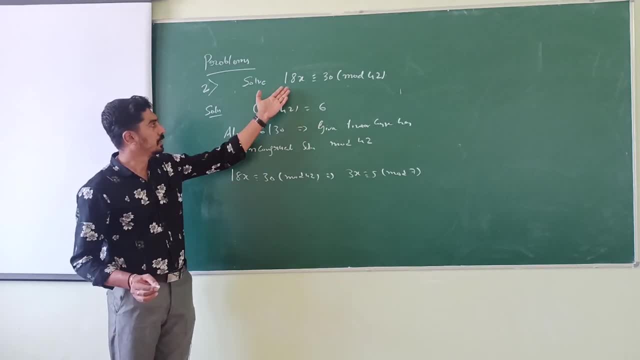 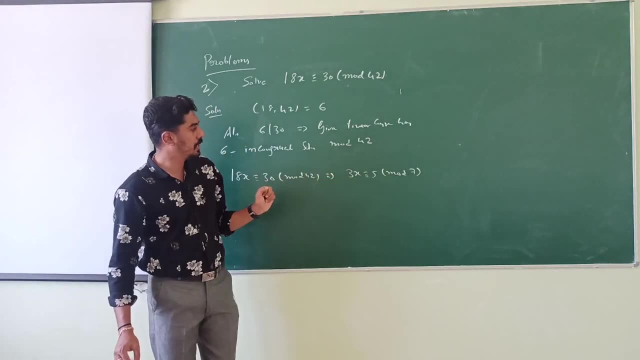 to find out a particular solution and later we can use this congruence to find out other solutions Here. in this case, by inspection, we can find out the solution for x equal to 1,. 3 minus 5, which is minus 2, is not a solution, is not a multiple of 7.. When I put x equal, 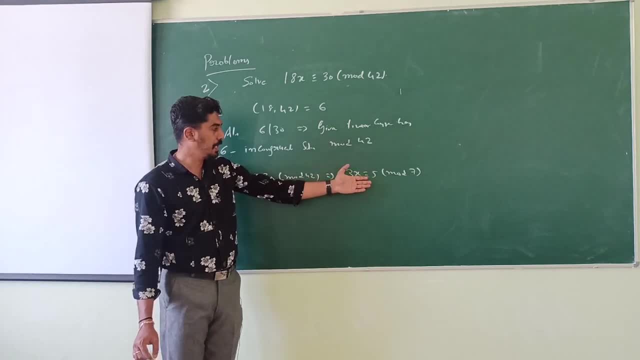 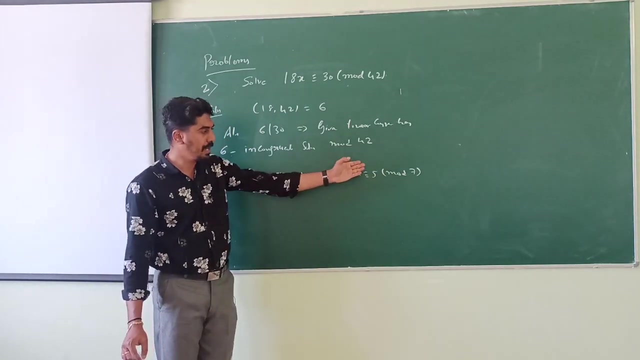 to 2, I get 6 minus 5, which is 1,. 1 is not a multiple of 7.. When I put x equal to 3,, I get 9 minus 5.. 9 minus 5, which is 4, is not a multiple of 7.. When I put x equal to 4,, I get 12 minus. 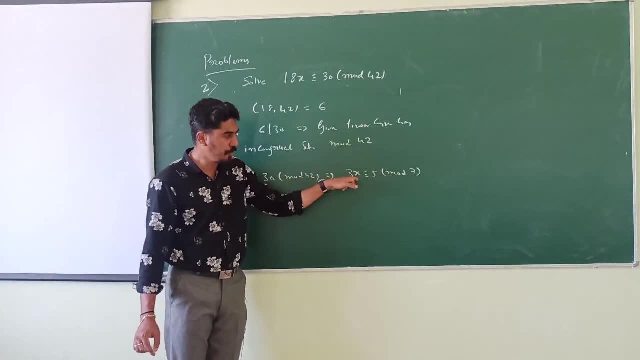 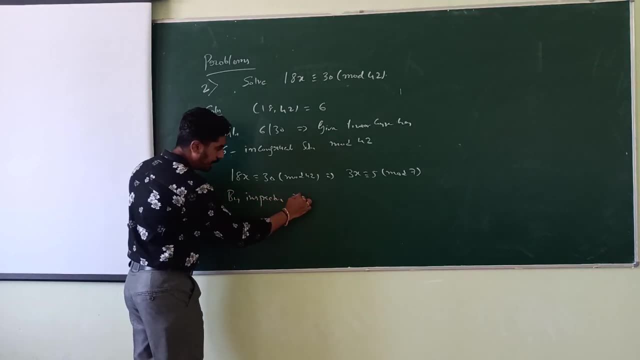 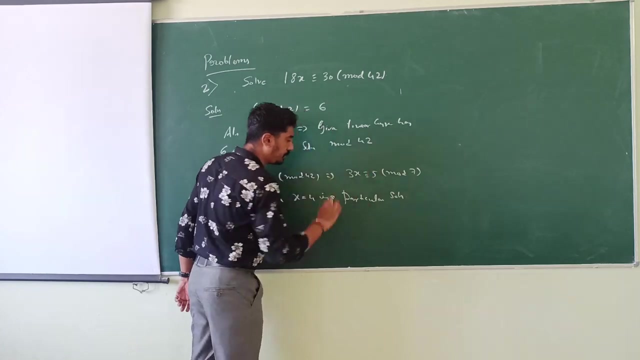 5, which is 7, is a multiple of 7. So x equal to 4 is a particular solution. By inspection x equal to 4 is a particular solution. Once we get a particular solution, then other solution we can find out easily. 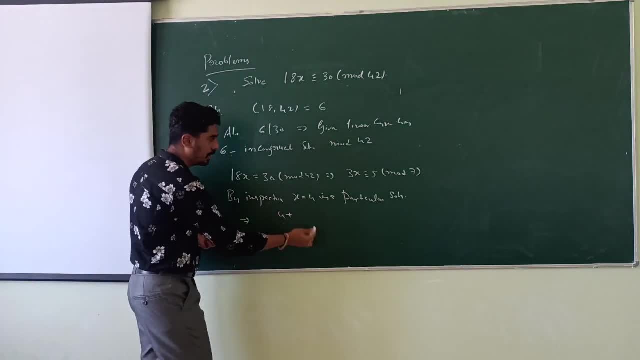 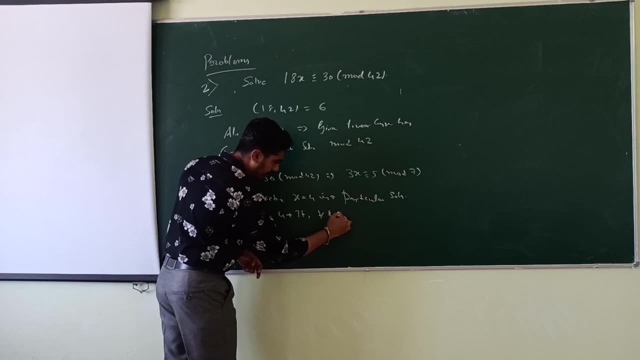 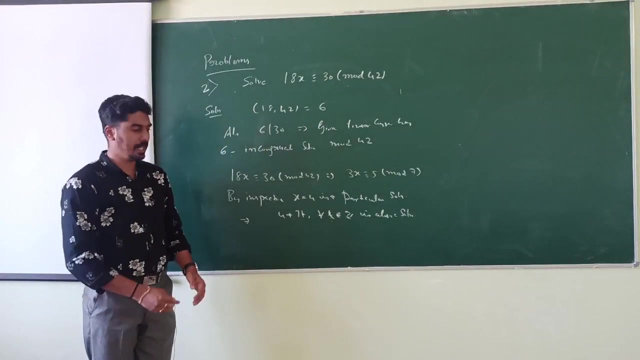 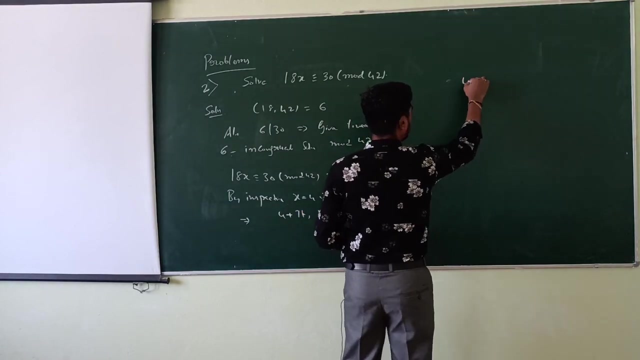 This implies that 4 plus 42 by 6, which is 7, t for all. t belongs to z is also a solution. To find out the incongruent solutions, I write down here: 4.. When I put t equal to 0, I get. 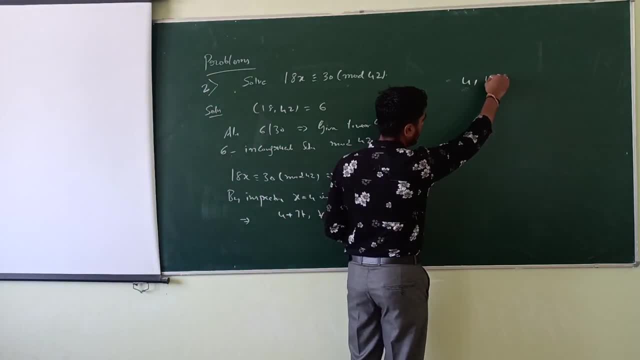 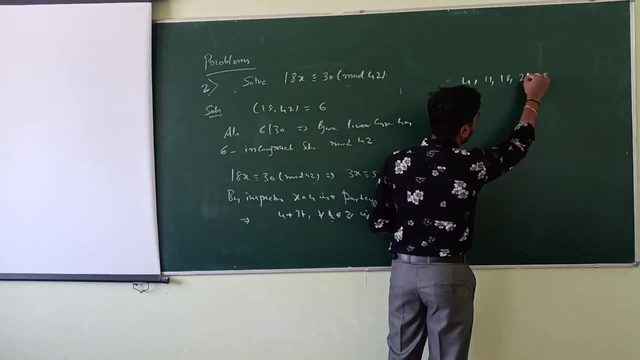 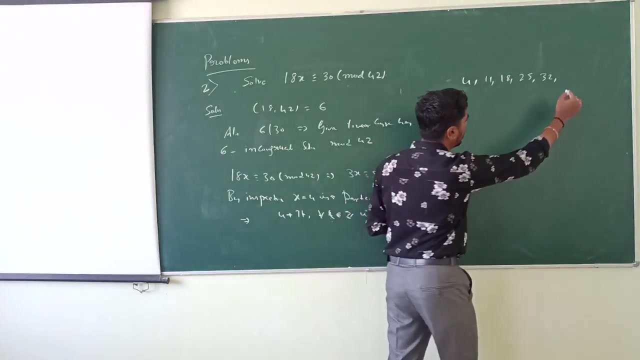 4. 4. 4 plus 7 is 11.. 11 plus 7 is 18.. 18 plus 7 is 25.. 25 plus 7 is 32.. 32 plus 7 is 39. So 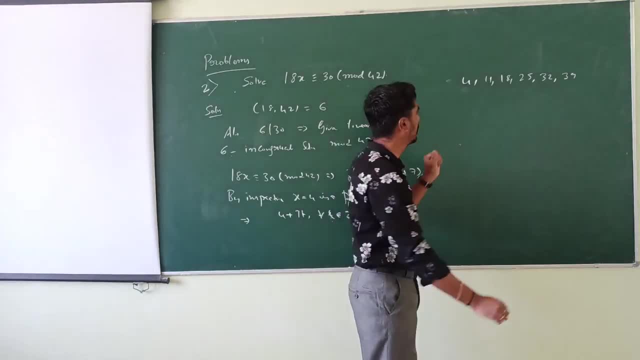 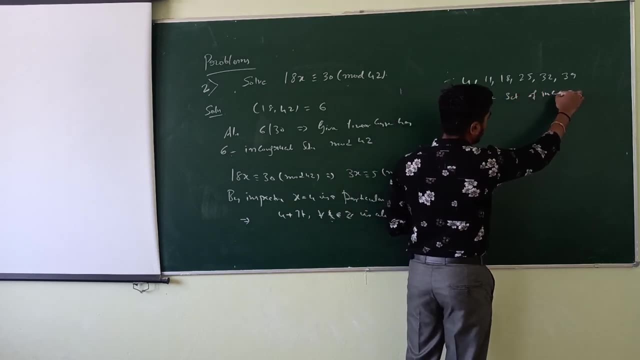 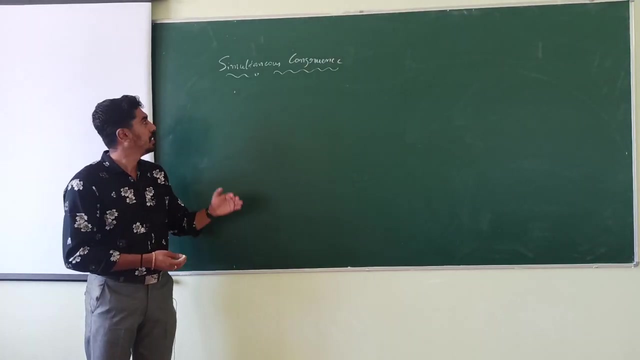 we have got 6 incongruent solutions is one set of incongruent solutions. berth Is less than or equal to 11.. Now let us discuss about simultaneous congruences. Consider a set of linear congruence: x congruent. 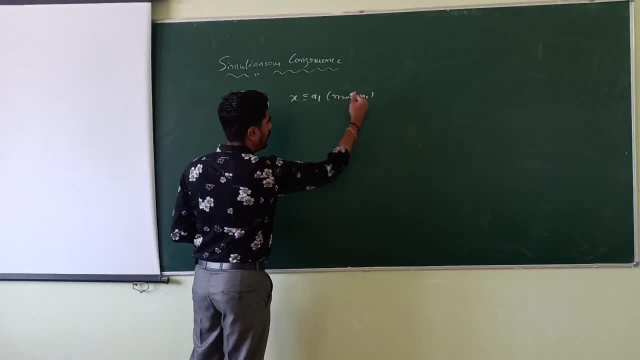 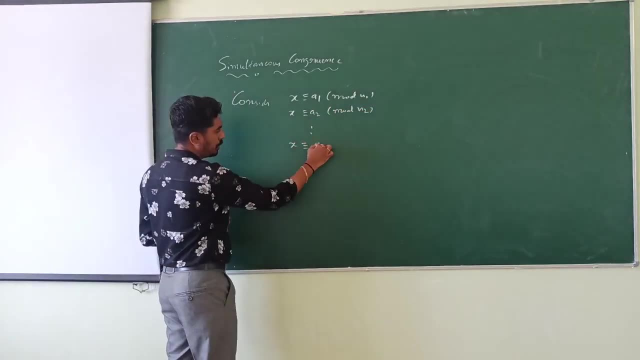 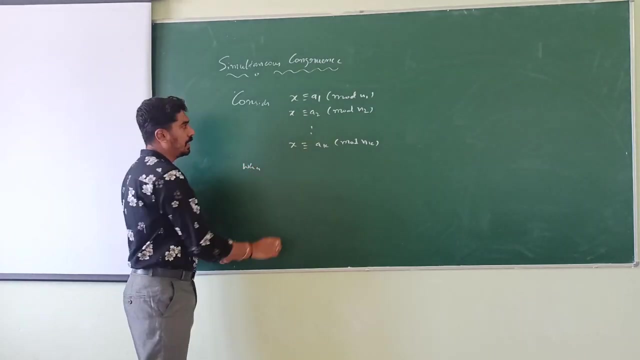 to a1 mod n1,, x congruent to a2 mod n2, and so on. x congruent to a k mod nk, where each where n1, n2, and nb are matchless In networks. x. congruent to x. congruent to a1 mode n1,. 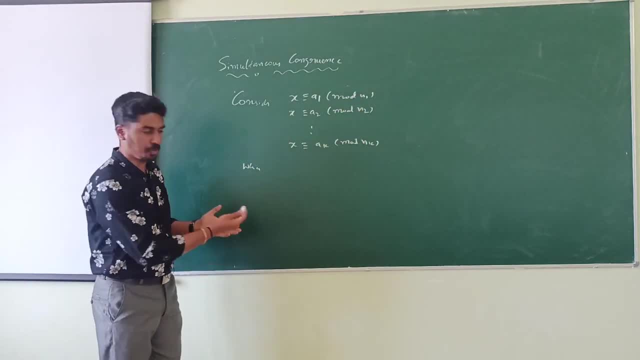 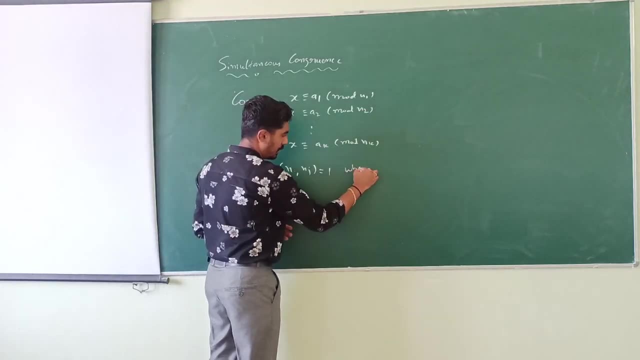 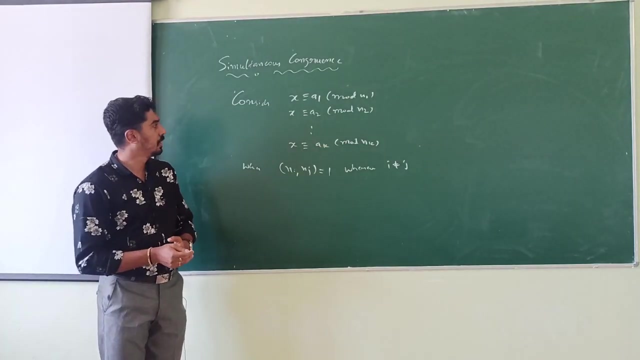 so on. So this aim is: nk are all mutually disjoint, that is, n i, n j. the gcd of n. i and n j is 1 whenever i not equal to g. first i am going to explain a method to find out a simultaneous solution for. 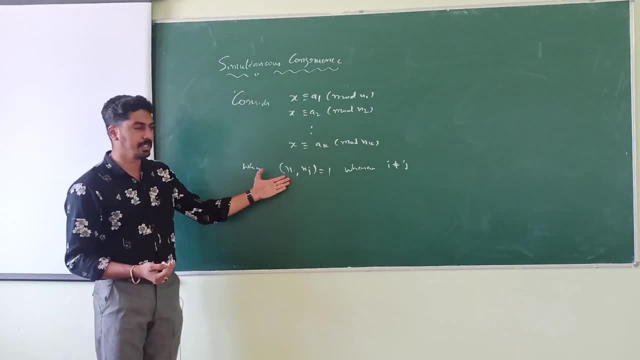 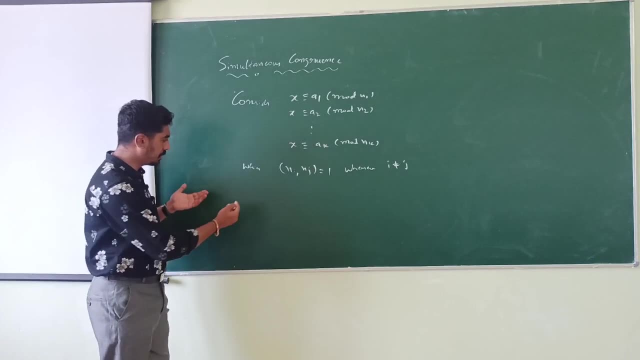 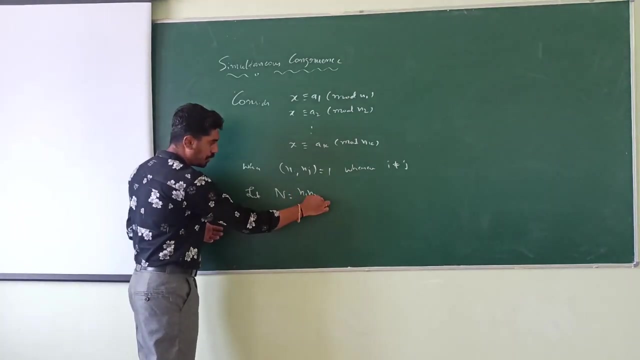 this set of linear concordance, satisfying this condition, which is well known as chinese remainder theorem. first, what we do is we consider the product of n1 into nk. let n be the product of n1, n2 and so on, and nk let define n1 by n, by n1. 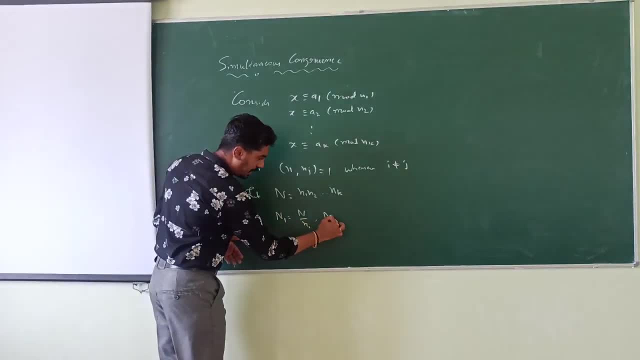 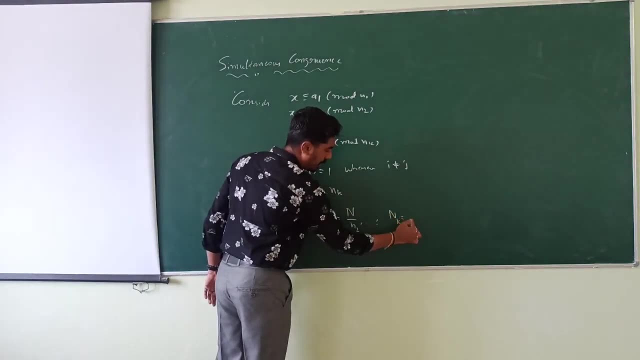 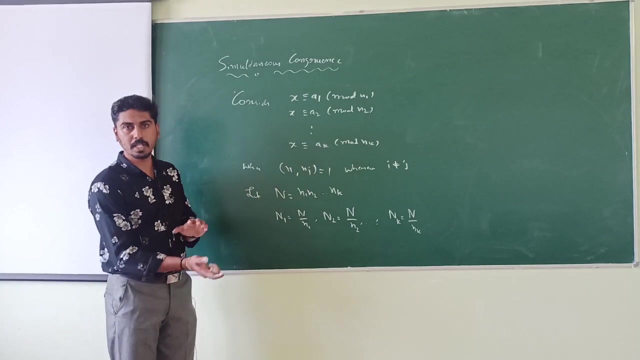 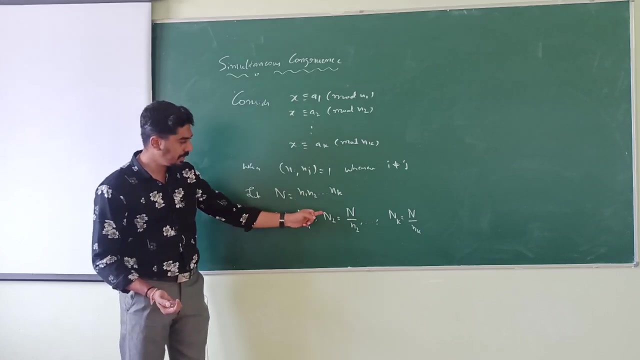 n2 by capital, n by n2, and so on, nk by capital, n by nk. we know that n1, n2, n, k are all mutually relatively prime. therefore n1 and small n1 are relatively prime. similarly, capital n2 and small n2 are relatively prime. 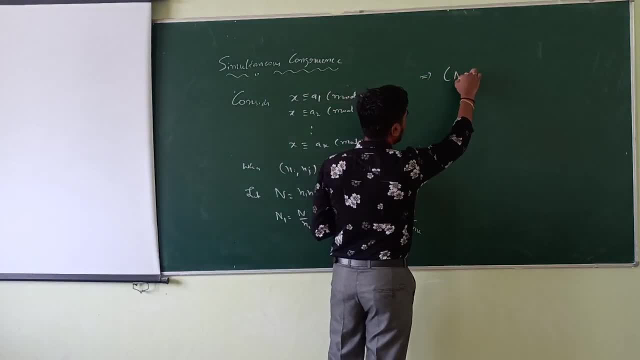 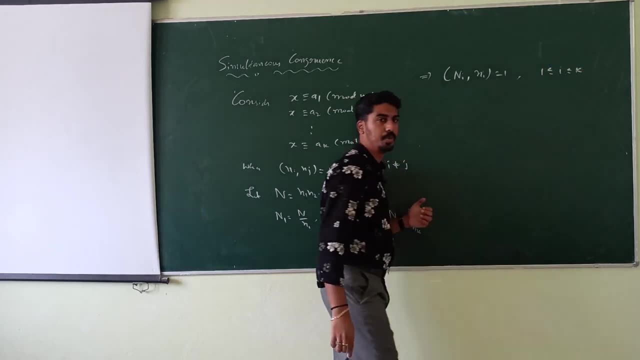 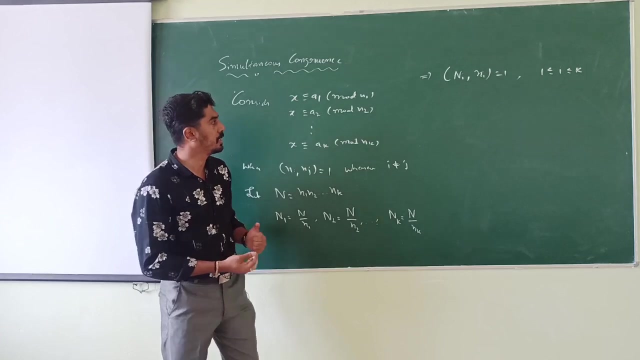 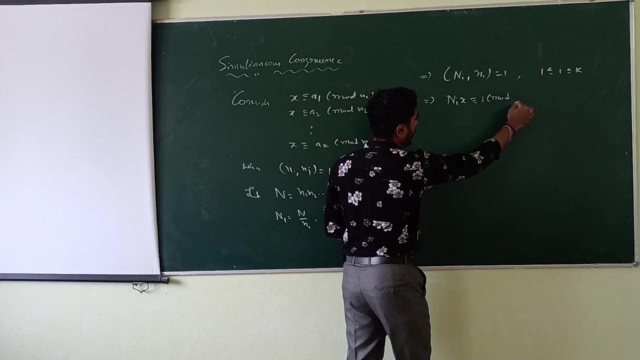 and so on. that is the gcd of n? i and small n i is 1 whenever i less than equal to k, greater than or equal to 1. now, using The property of linear congruence, we know that n i x congruent to 1. modulo n i has a. 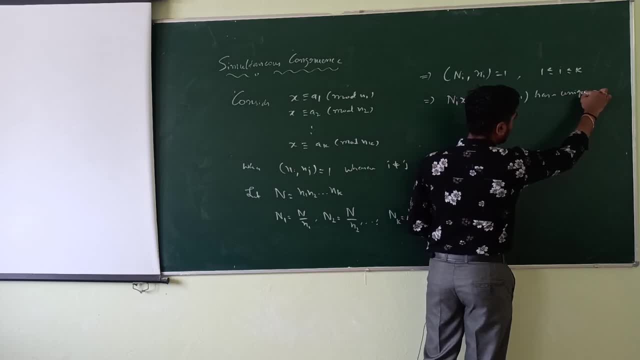 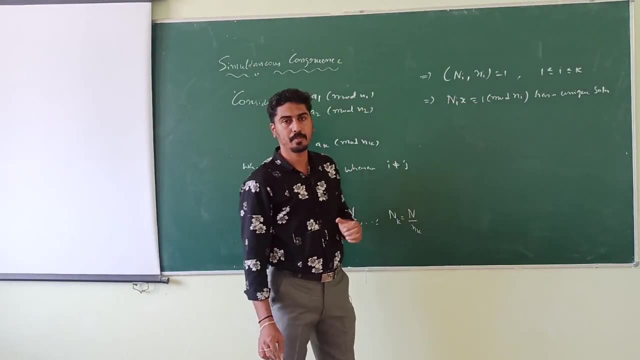 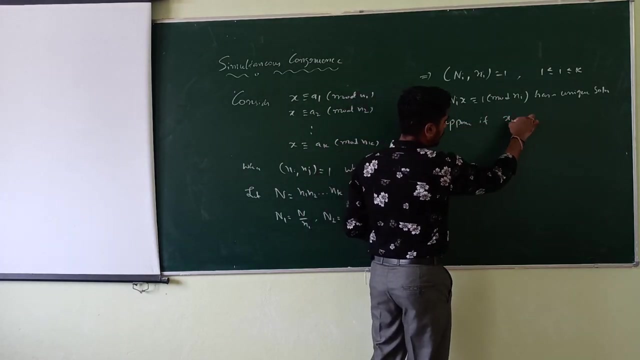 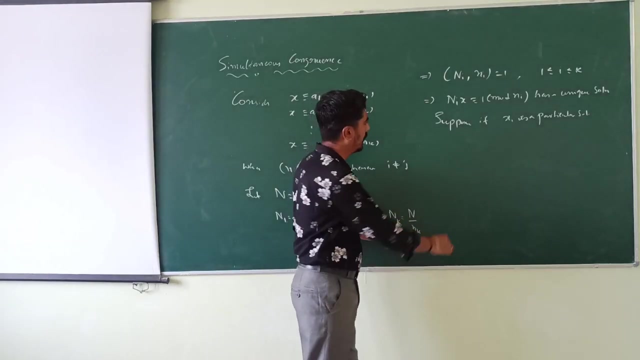 unique solution. Since the GCD of n? i and n? i is 1 and 1 divides 1, it has a unique solution. Suppose if x- 1 is a particular solution, then we have n? i into x. i is congruent to. 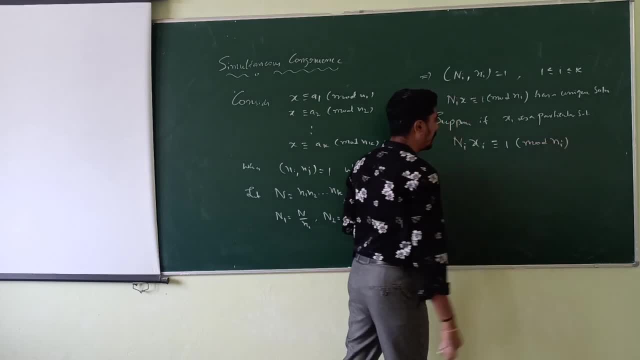 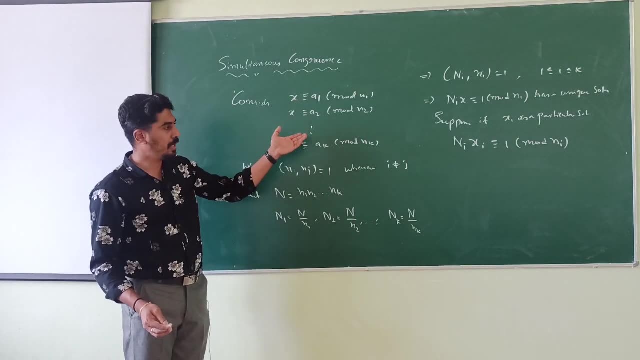 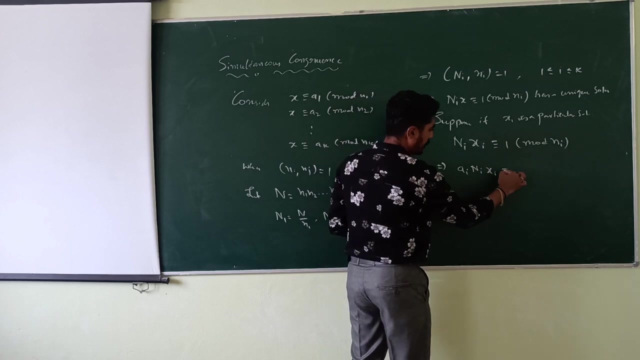 1 mod n i, where i between 1 and k. To get a solution for this congruence, I multiply both sides. I multiply a i. This implies a i n i, x. i is congruent to a i mod n i. So we have got. 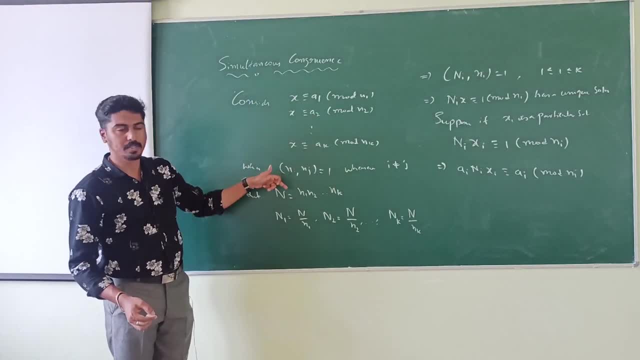 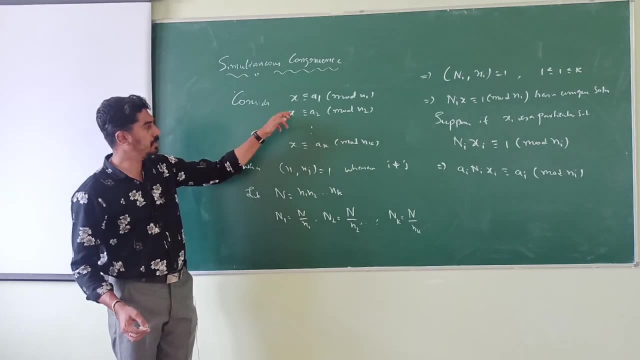 a solution for these congruences. For the first congruence, a 1 n. 1 x 1, is a solution. For the second congruence, a 2 n, 2 x 2 is a solution, and so on: a, k, n, k, x, k is a solution. 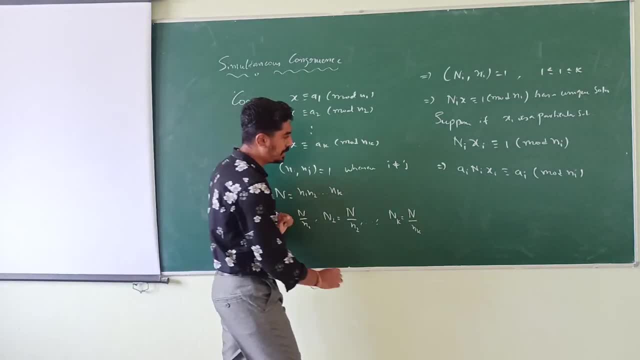 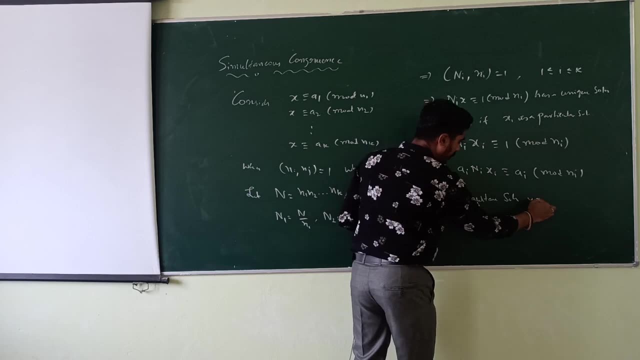 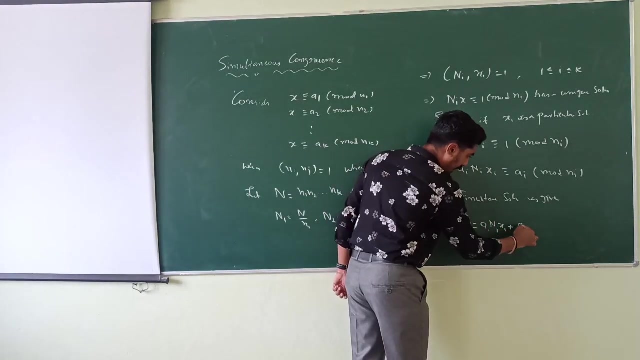 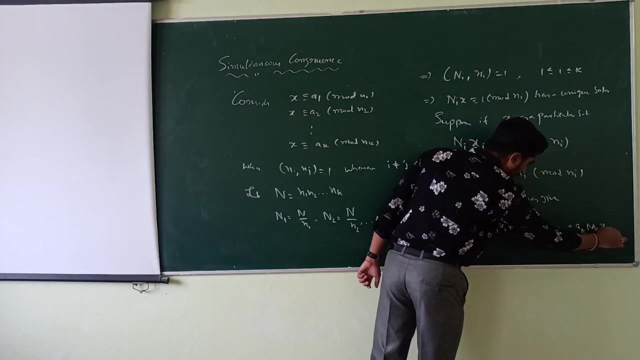 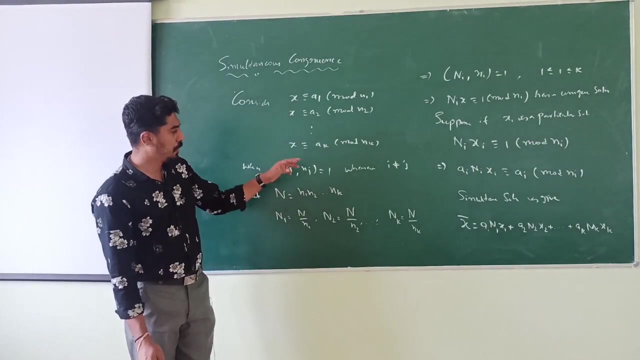 for this congruence. So the simultaneous solution is given by x bar is equal to a 1 n 1 x 1 plus a 2 n, 2 x 2, and so on: a k, n, k, x k. I will explain with an example how this works. Suppose if 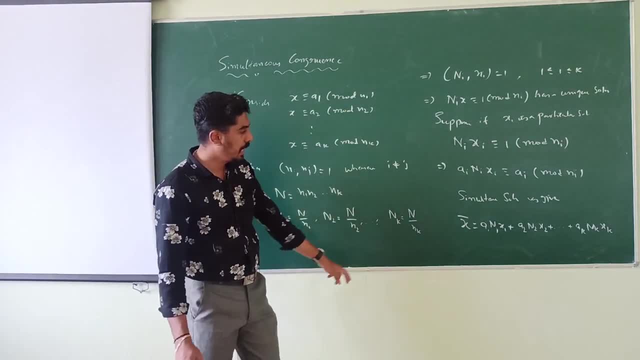 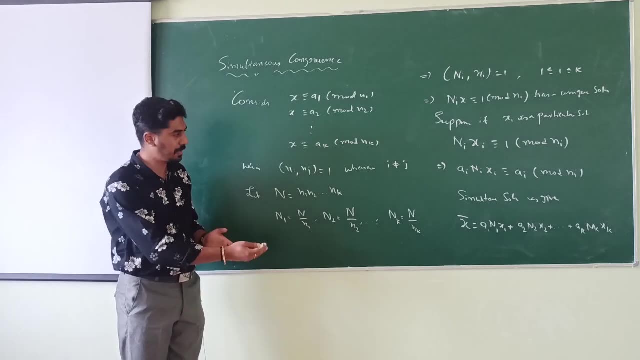 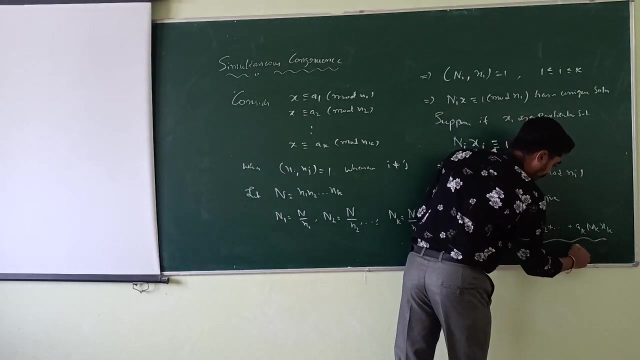 I take x bar modulo n 1,. in the first term we do not have n 1,, since n 1 and small n 1 are relatively prime. But in all other terms we have n 1.. So these are all becomes 0 and 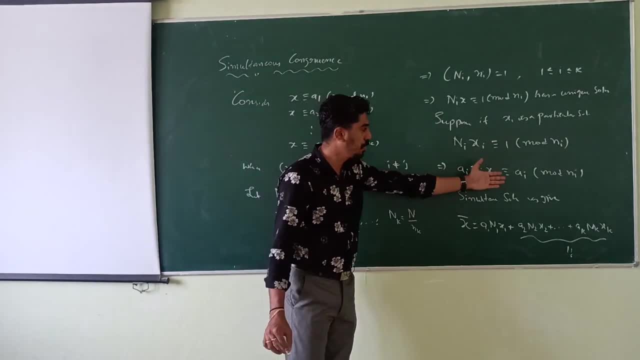 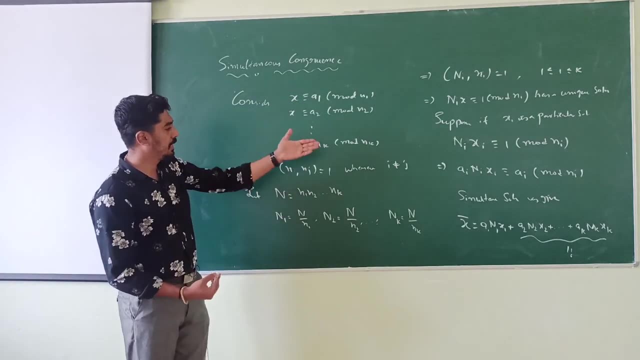 we remain with a 1 n, 1 x 1, which is congruent to a 1 mod n, 1.. So x bar is a solution for first congruence. Similarly, I can show that it is a solution For second congruence, and so on a solution for last congruence. So this is a simultaneous 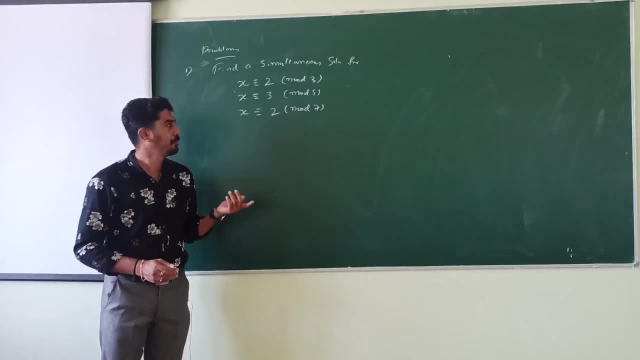 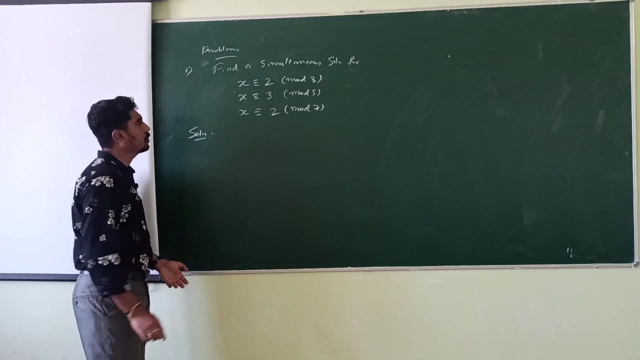 solution. Now let us consider a problem. Find a simultaneous solution for the congruences x congruent to 2 modulo 3, x congruent to 3 modulo 5, x congruent to 2 modulo 7. solution: First consider the congruence. 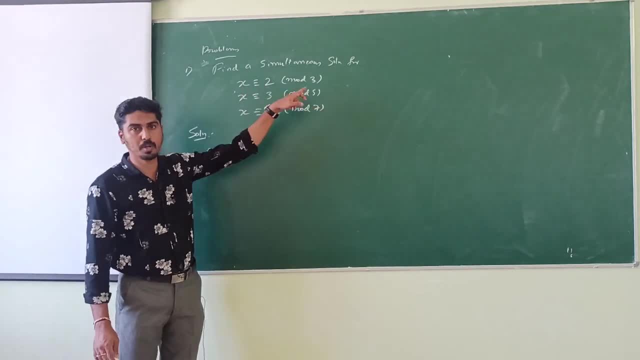 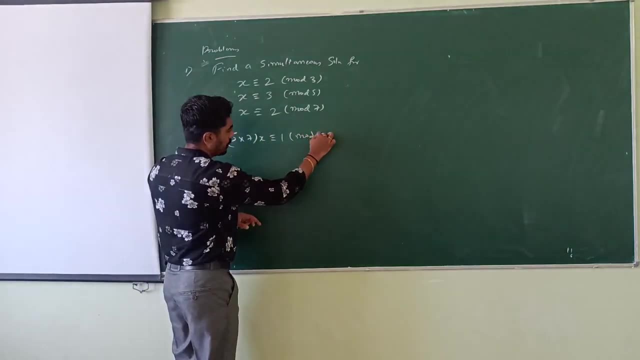 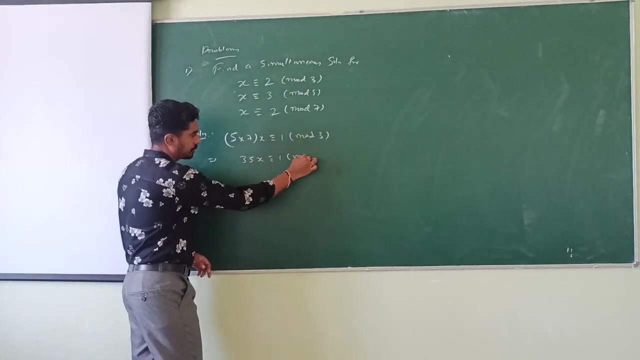 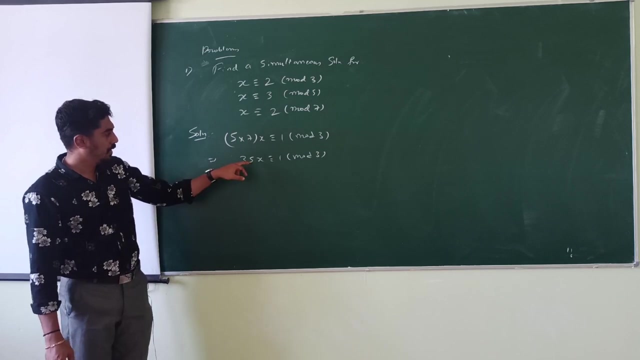 5 into 7 x, congruent to 1 modulo 3,. 5 into 7 x, congruent to 1 modulo 3, which is 35 x congruent to 1 modulo 3.. By inspection, x equal to 2 is a solution If I put x equal. 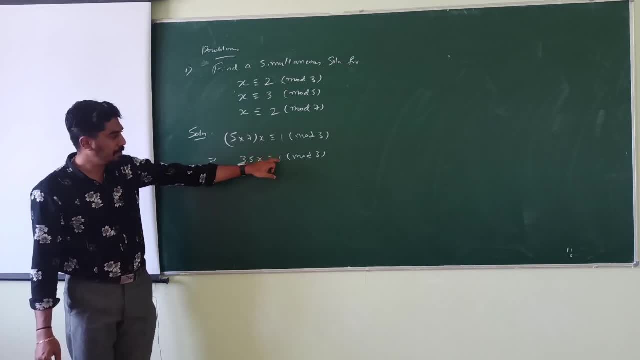 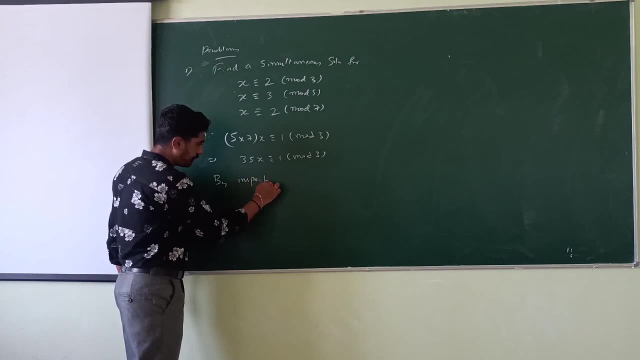 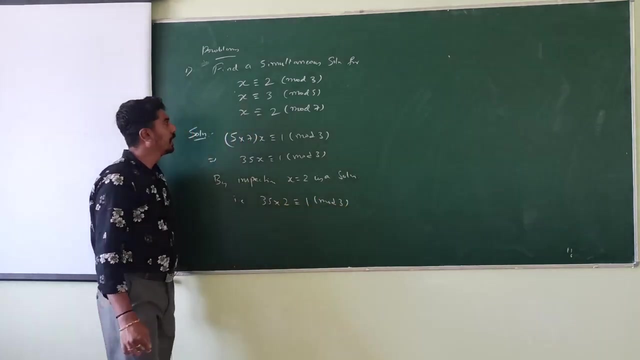 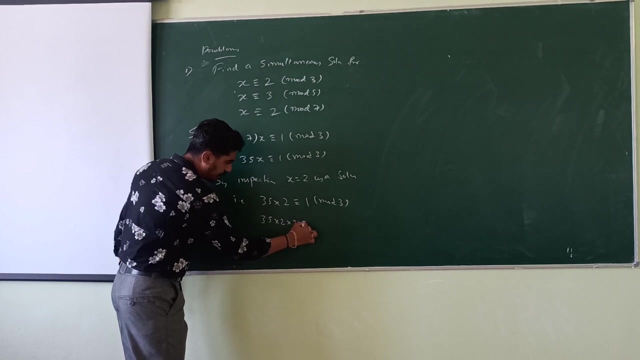 to 2, we get 35 into 2 is 70.. 70 minus 1. 70 is 75.. Very nice: 55,, which is very Mi, plus 9.. Very nice, It is important It has 30, because that is NO asaxis. 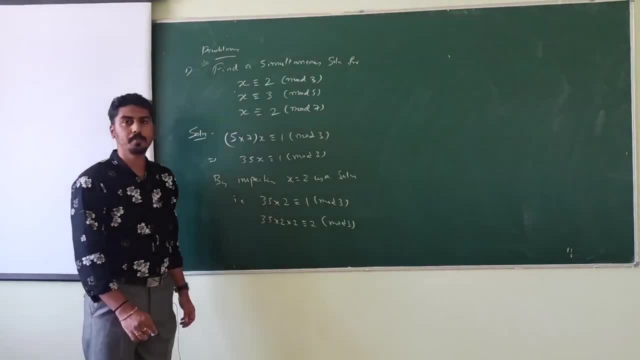 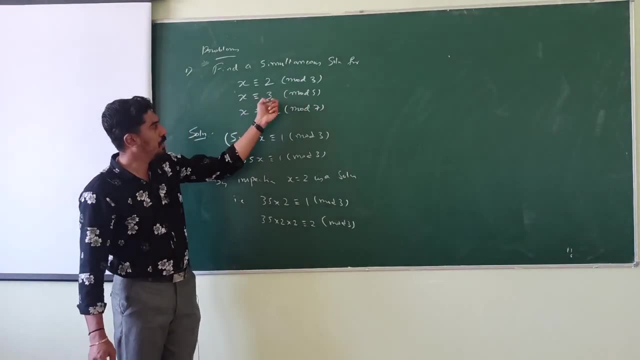 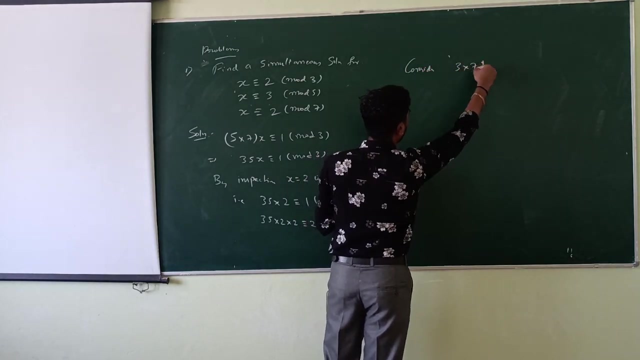 There is no minus. seesaw There is no minus. the stressor There is no plus. if There is a lac decentralization here, Recall that Ops. Now let us consider the congruence 3 x 7x congruent to 1 modulo 5.. Consider 3 x 7x congruent. 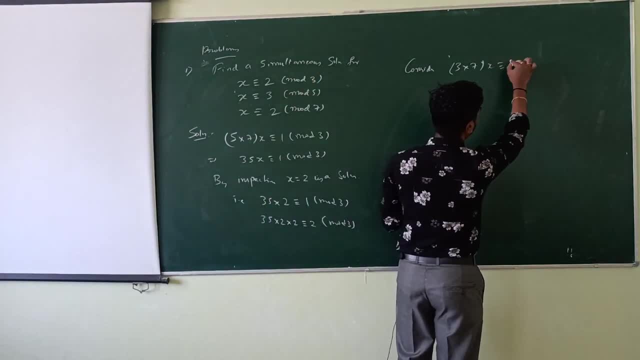 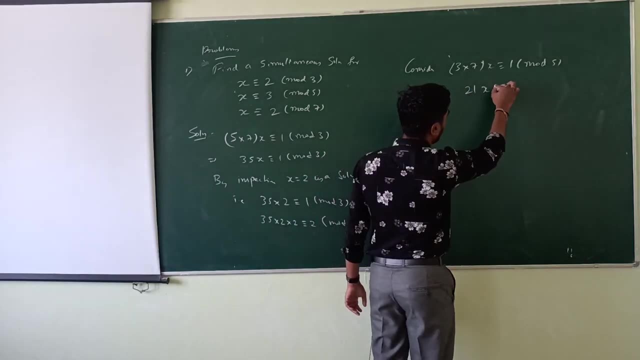 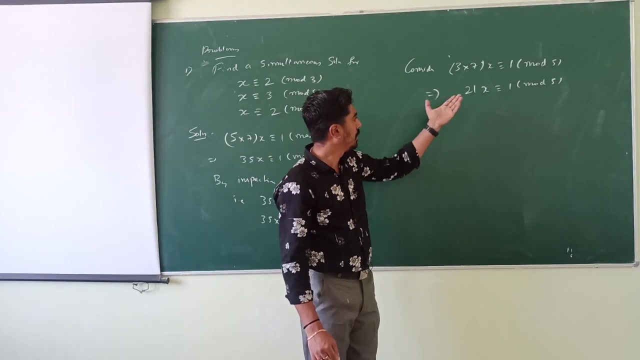 to 1 modulo 5, which is same as 21 x congruent to 1 modulo 5.. By inspection, we see that x equal to 1 is a solution. When I put x equal to 1, we get 21 minus 1, which is 20 is a multiple. 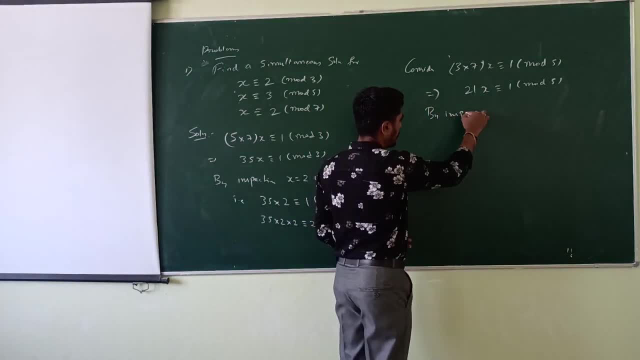 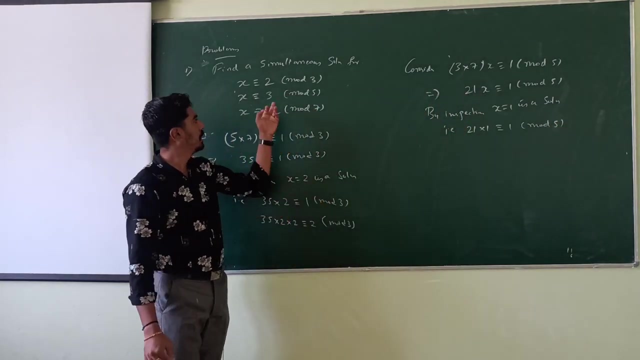 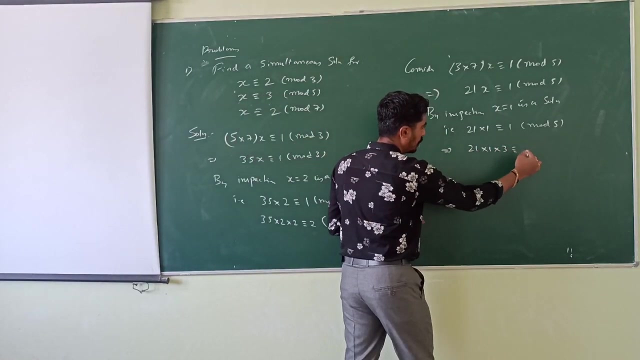 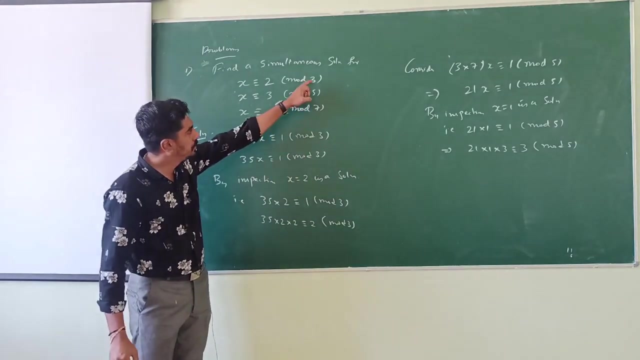 of 5.. By inspection, x equal to 1 is a solution. That is, 21 into 1 is congruent to 1 modulo 5.. I have 3 here, so multiply both sides by 3. We get 21 into 1. into 3 is congruent to 3 modulo 5.. Finally, consider 3 into 5, x congruent. 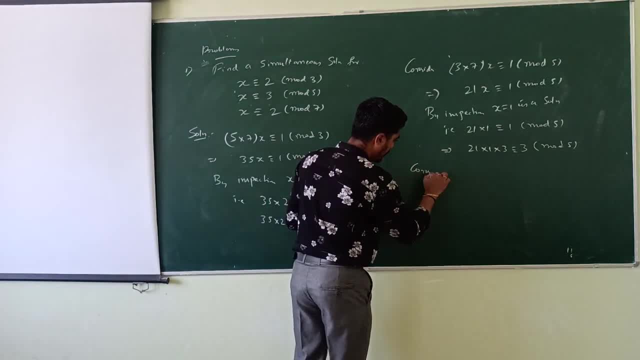 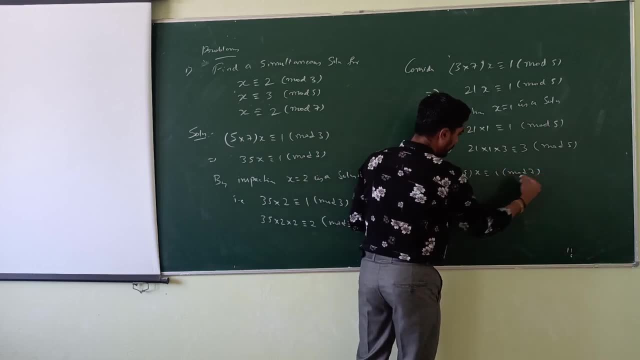 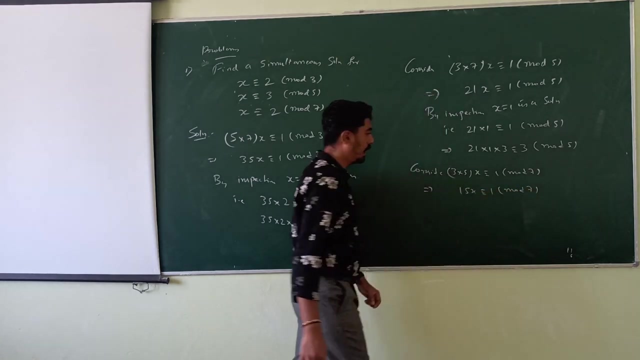 to 1 modulo 7.. Consider 3 INTO 5 x congruent to 1 modulo 7, which is same as 15 x congruent to 1 modulo 7.. By inspection we see that x equal to 1 is solution. 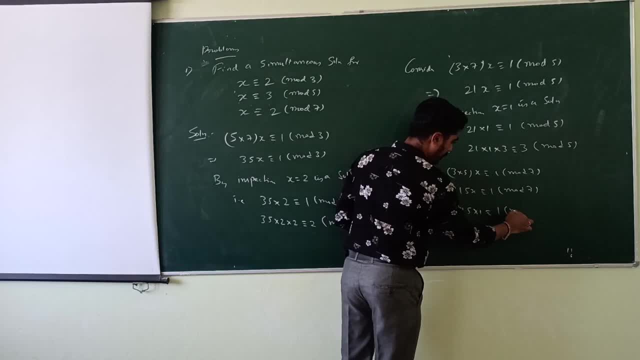 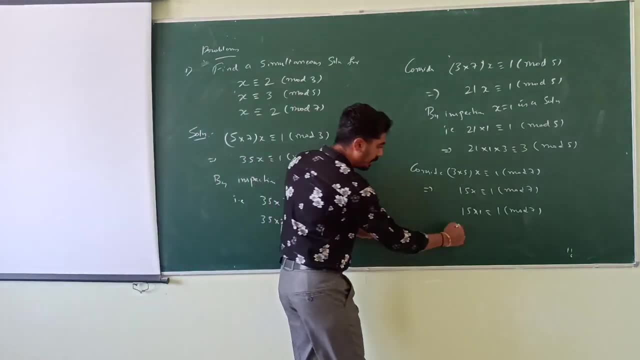 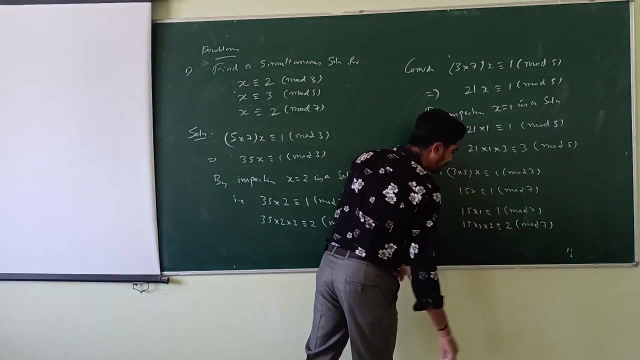 So 15 into 1 is congruent to 1 modulo 7.. Here I have two. so multiply both sides by 2.. 15 into 1 into 2 is congruent to 2 modulo 7. So the simultaneous solution is sum of: 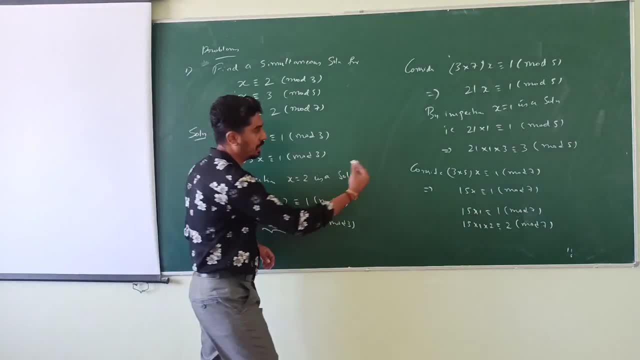 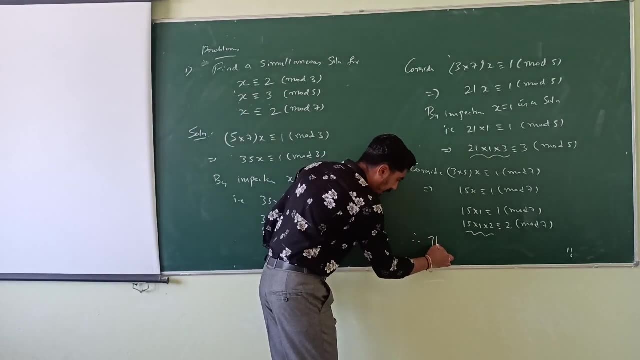 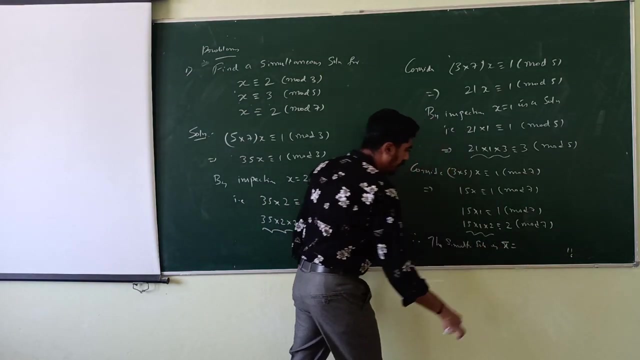 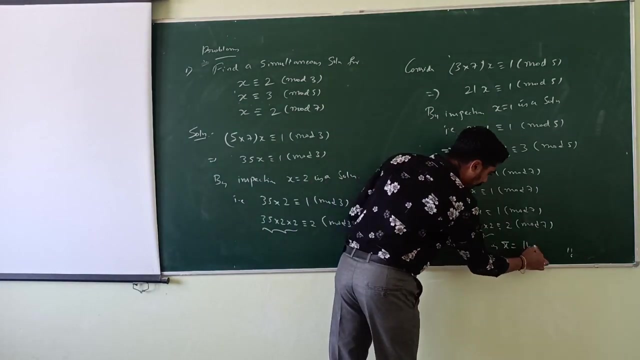 35 into 2 into 2, plus 21 into 1 into 3, plus 15 into 1 into 2.. Therefore, the simultaneous solution is: x. bar is equal to 35 into 2 into 2, which is 140, plus 21 into 3, which is 63. 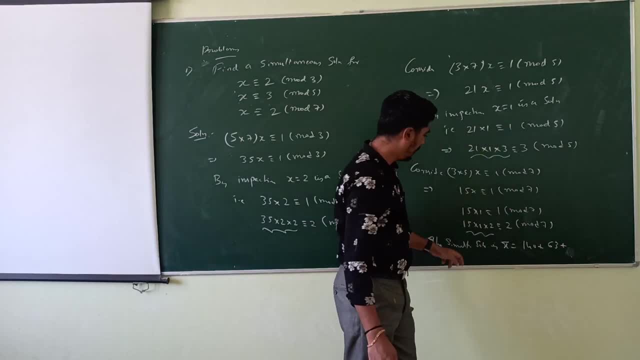 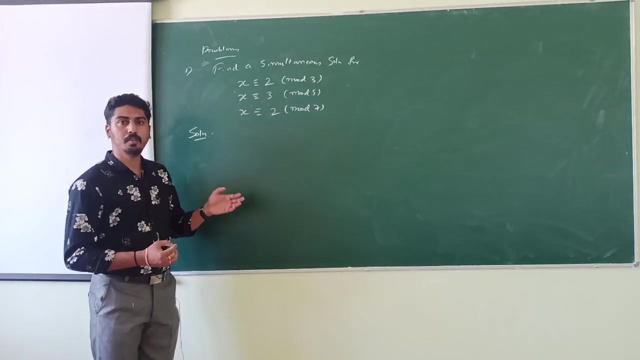 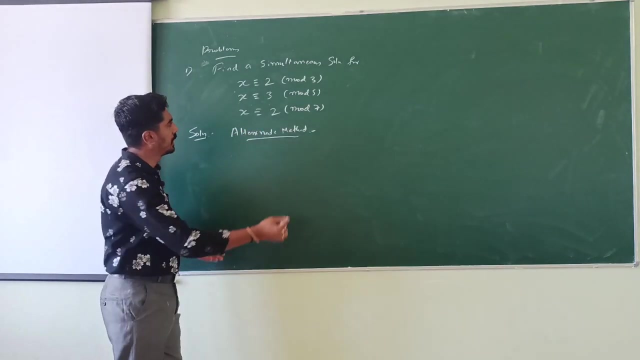 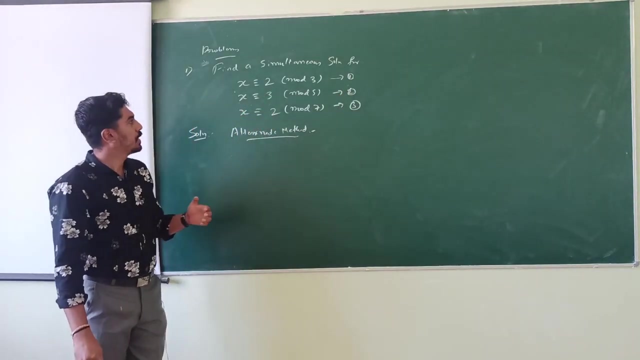 plus 15 into 2, which is 30.. So the simultaneous solution is 233.. We have one more method of solving this problem, alternate method. First, what we do is: I consider this congruence as 1, this as 2 and this as 3.. We can find out a solution for this congruence. 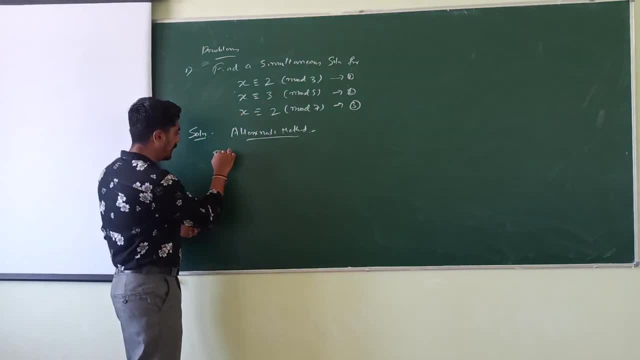 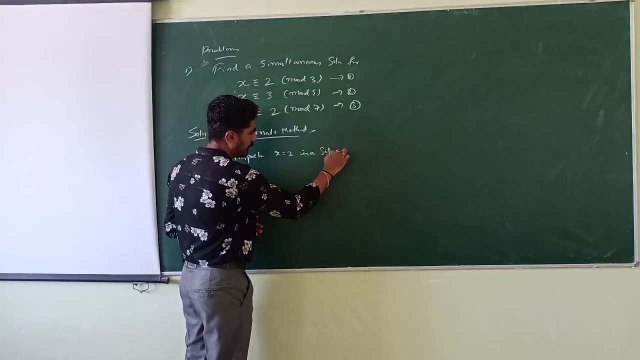 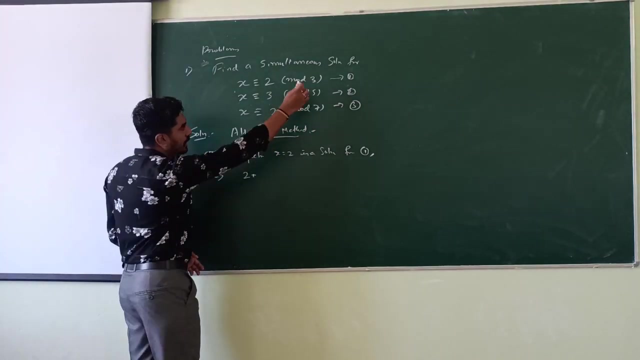 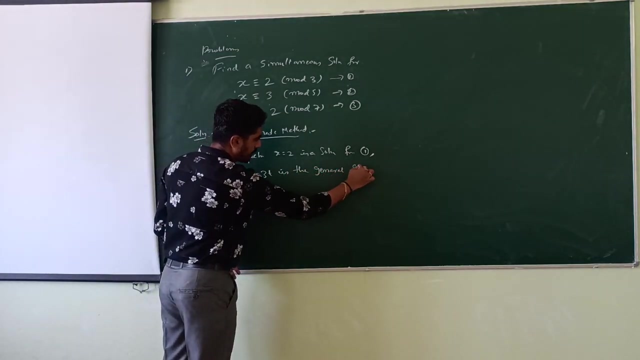 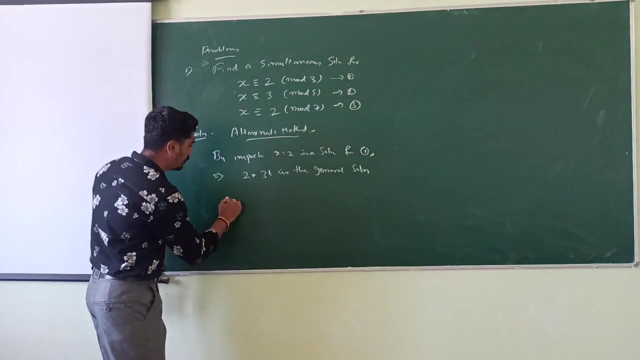 by inspection, x equal to 2 is a solution. By inspection, x equal to 2 is a solution. 2 is a solution for 1.. So 2 plus 3t is the general solution. Now substitute this in equation 2, put x equal to 2 plus 3t in 2.. 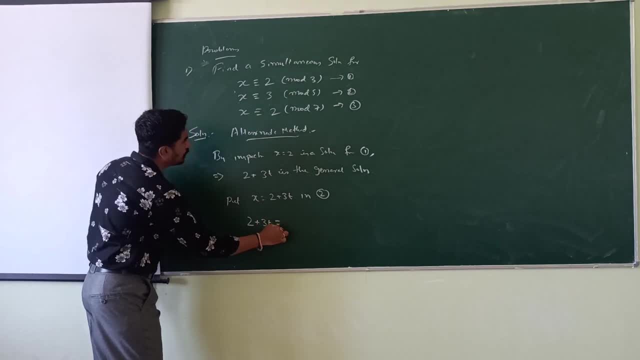 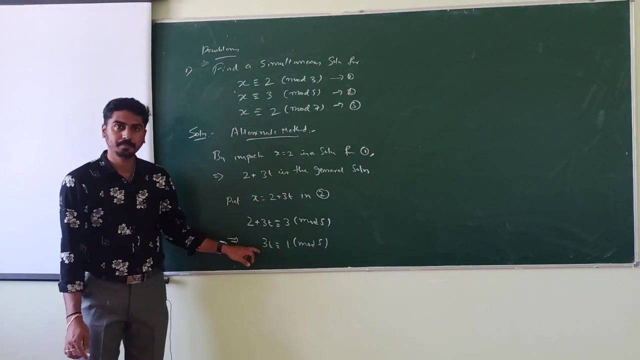 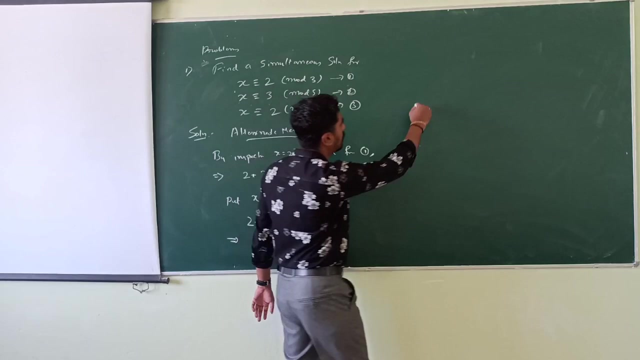 2 plus 3t, congruent to 3 modulo 5, which is same as 3t congruent to 1 modulo 5.. Now find out a solution by inspection. I see that t equal to 2 is a solution By inspection. t. 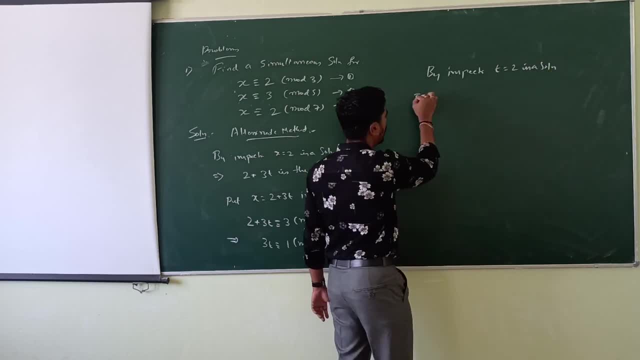 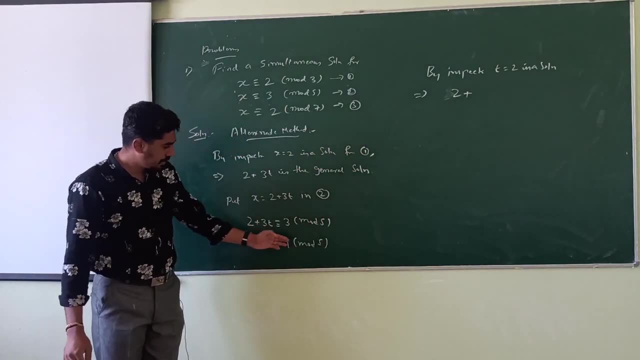 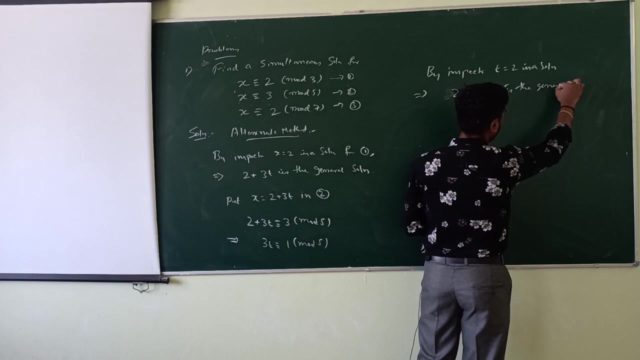 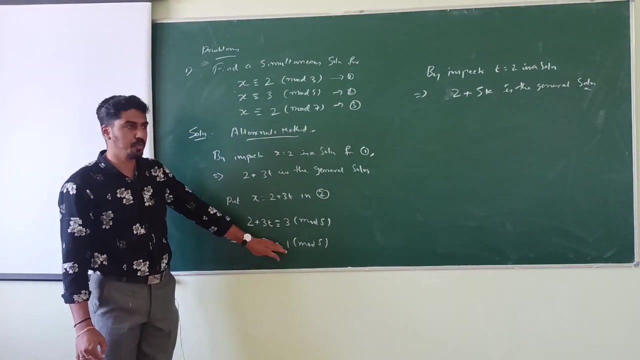 equal to 2 is a solution, So 2 plus 3t is the general solution. Now substitute this solution And therefore 2 plus 5k is a general solution, So 2 plus 5k is the general solution. 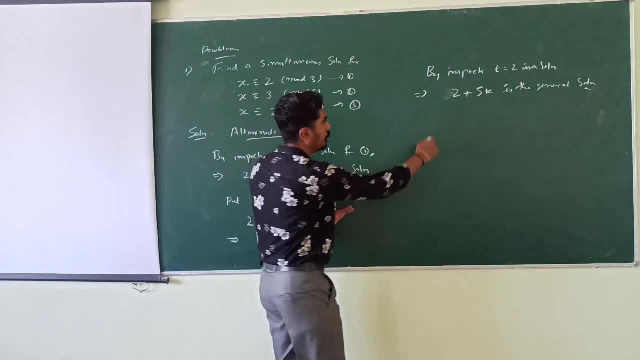 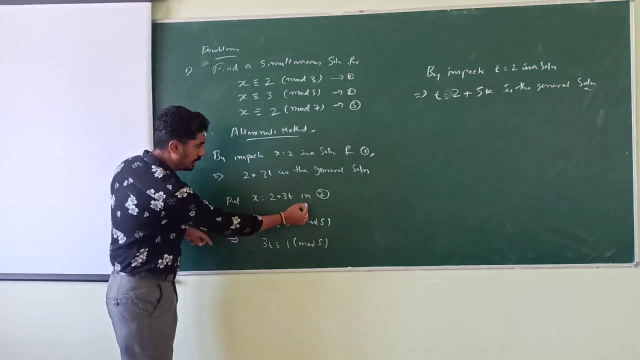 for this congruence t equal to 2 plus 5k. When I substitute 2 plus 5k for this congruence t equal to 2 plus 5k to this one, I get a simultaneous solution for first and second. 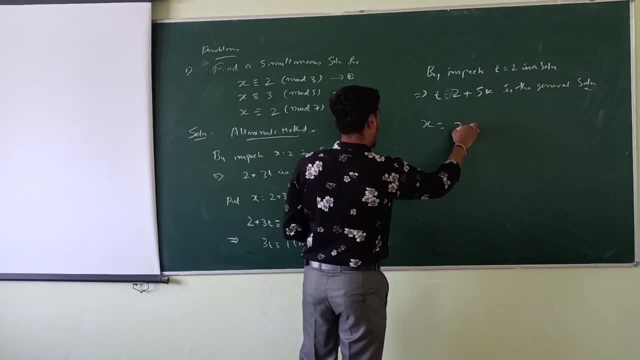 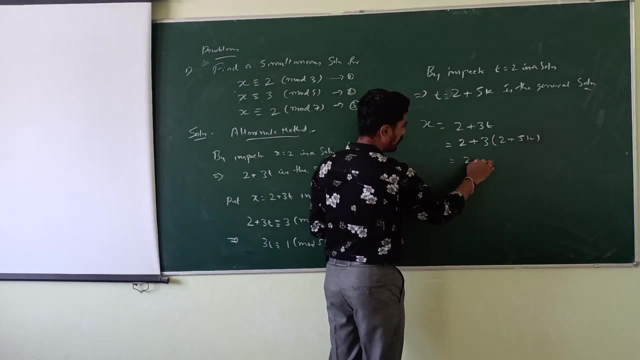 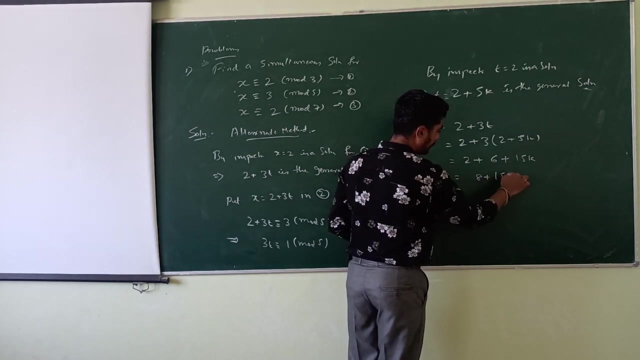 congruence. Therefore, x equal to 2 plus 3t is equal to 2 plus 3 into 2 plus 5k, which is same as 2 plus 6 plus 15k, or 8 plus 15k is the general solution. So this is the general. 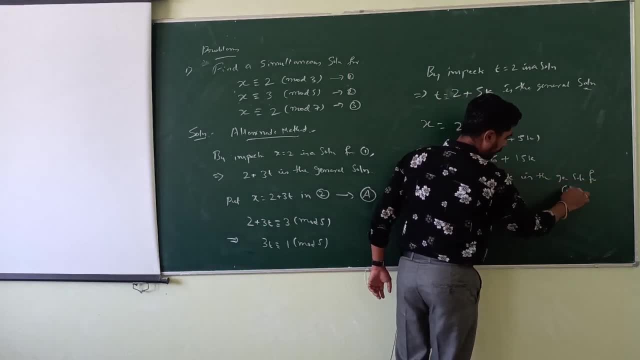 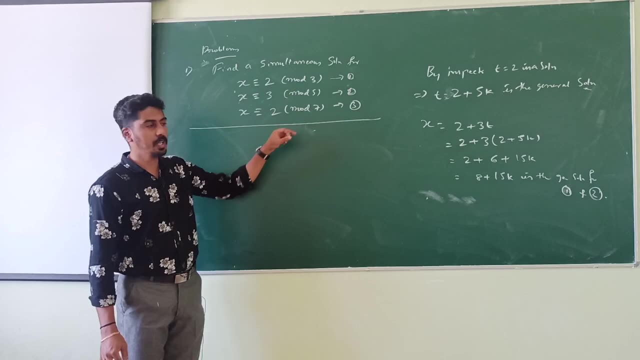 solution for 1 and 2.. Now we have got simultaneous solution for 1 and 2.. To find out the simultaneous solution for 1, 2 and 3, substitute x equal to 8 plus 15k in the third congruence Put. 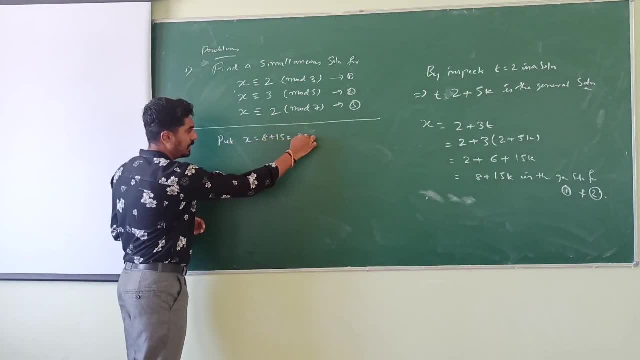 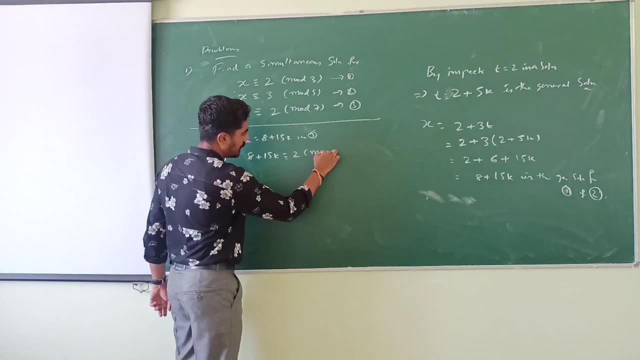 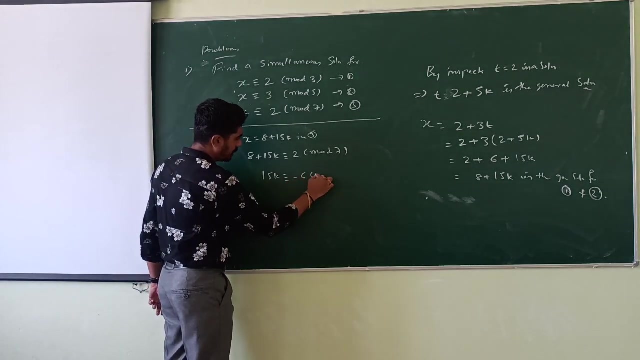 x equal to 8 plus 15k in 3. We get: 8 plus 15k is congruent to 2 plus 5k. So this is congruent to 2. modulo 7 or 15k is congruent to minus 6. modulo 7 or 15k is congruent to: 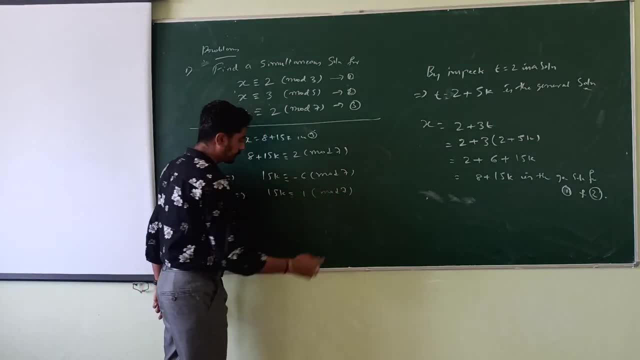 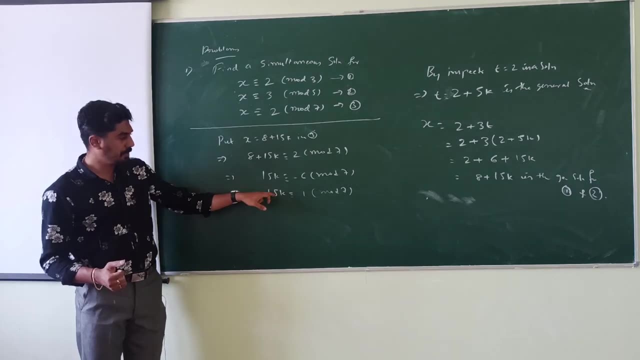 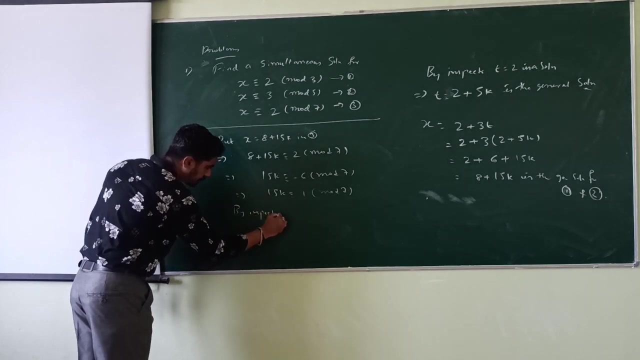 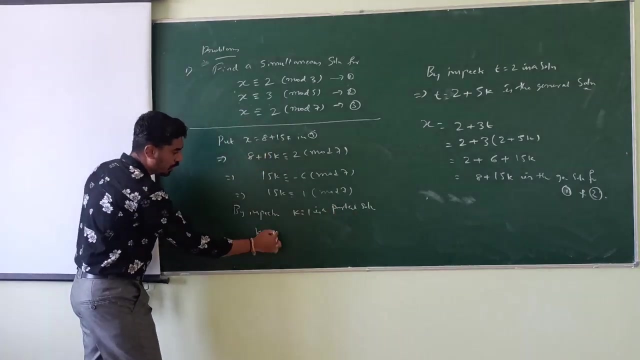 1 modulo 7.. By inspection I see that k equal to 1 is a particular solution. I get 15 minus 1 is a multiple of 7.. By inspection, k equal to 1 is a particular solution. So k equal to 1 plus 7m for all. 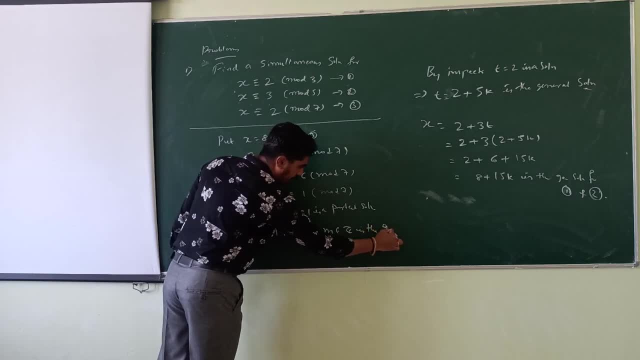 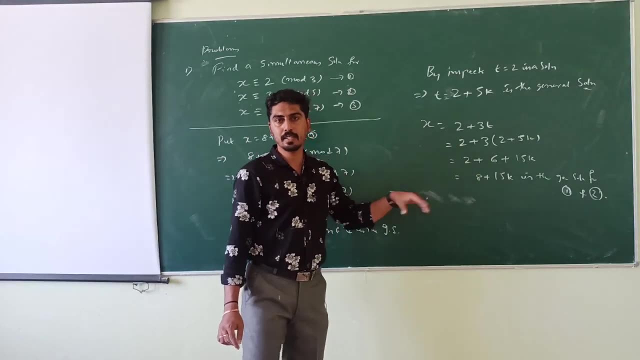 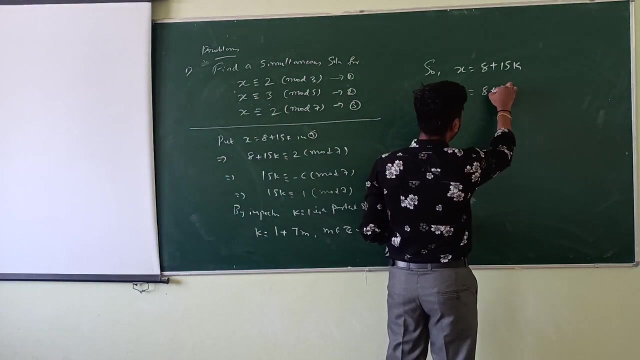 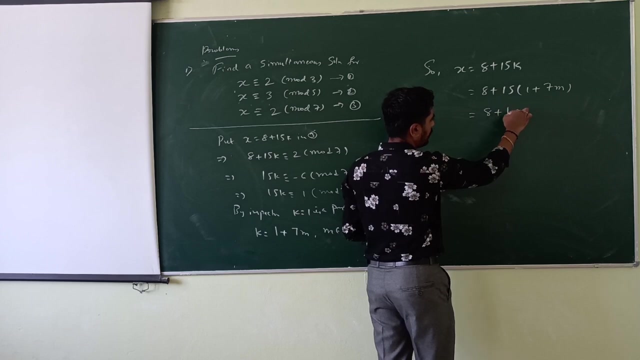 m belongs to. z is the general solution. Now I am going to substitute this in this to get the simultaneous solution. Now substitute k equal to 1 plus 7m In x equal to 8 plus 15k. we get 8 plus 15 into 1 plus 7m, which is same as 8 plus 15. 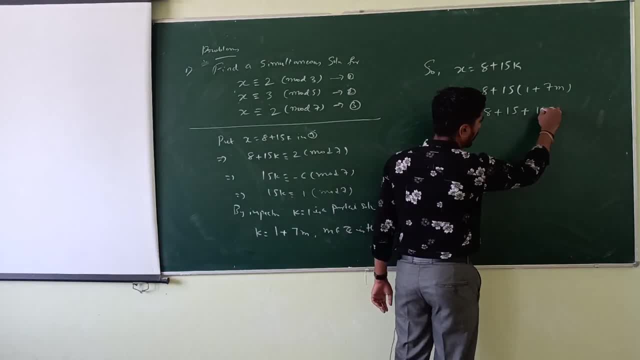 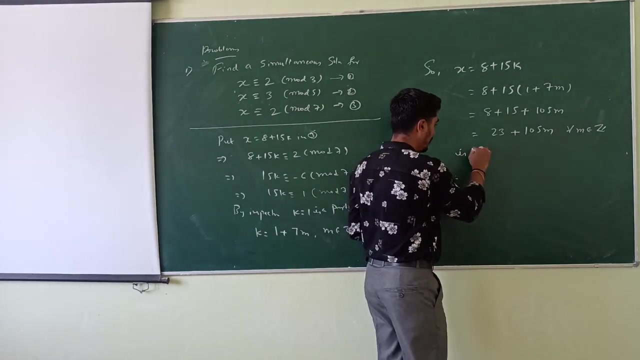 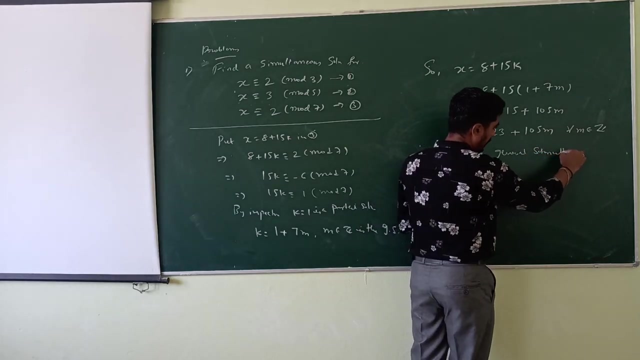 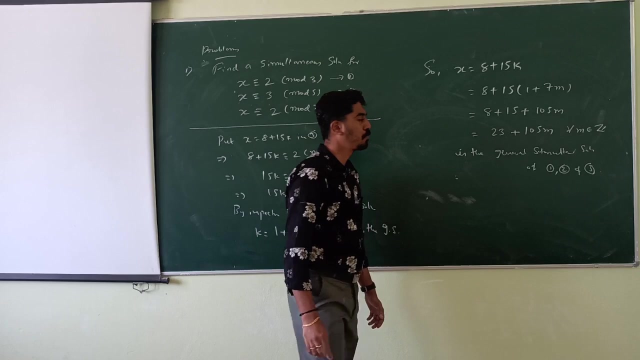 plus 1 naught 5m, or I get 23 plus 1 naught 5m, for all m belongs to z is the general solution for is the general solution general simultaneous solution of 1, 2 and 3.. As we have found earlier when 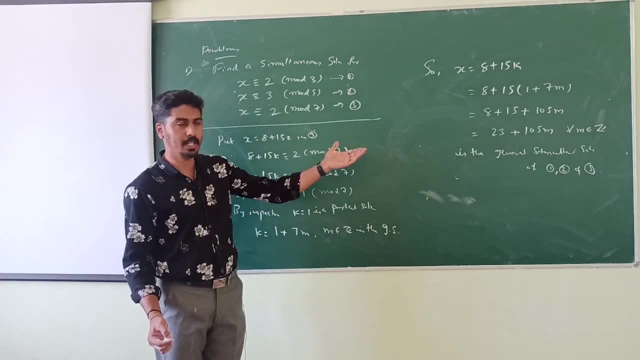 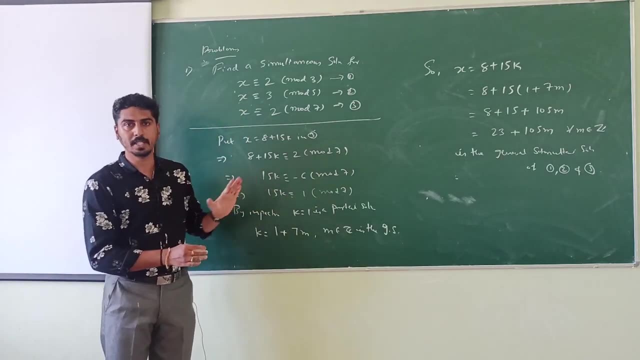 I put m equal to 2, I get 210 plus 23,, which is 233 is a particular solution. So this gives the general solution, this method To find out a particular solution. we have to think first about how we are going to find out an angle in this particular function. So now a multiple of time constraint. Eve. We are putting a multiple, so I have to try and justify this. So take the half a- that means 10 times the length of vector, to say, into discern 1 over 4 times, and the last difference is 10t, all this times by 2.. So what I need to find is: 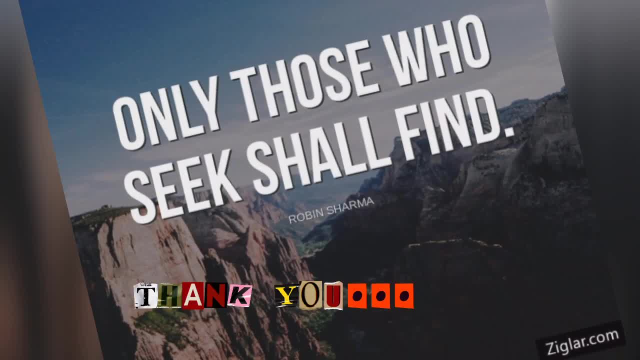 just this big value that is plus 0.. Ok, So this is what I am going to represent here by this doubleuntu, and I want to use some naked number. We can use many comma minus 1, this whole equation letter, because this becomes a binary.